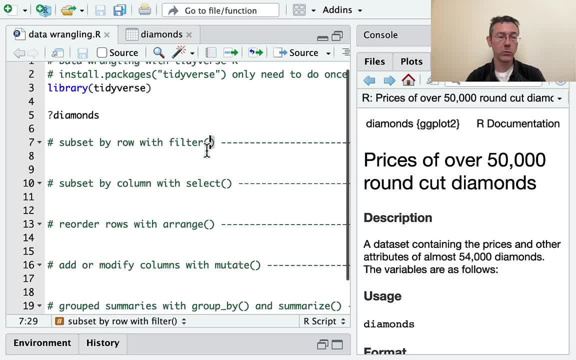 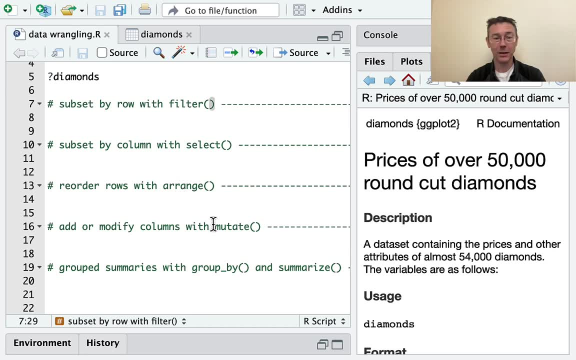 going to show you how to do all of those things. We're going to subset by rows and by columns, with filter and select respectively. We're going to reorder rows with arrange. We're going to modify columns or add new columns with mutate, And then we're going to handle. 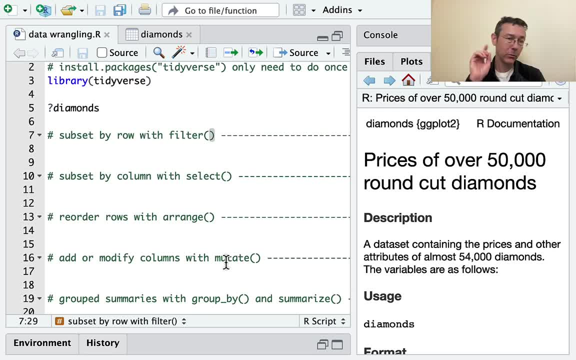 some group summaries. I'll throw up some links to some longer form videos on some of these topics that I've already done And I'll also give you just some signposts for some additional areas of exploration, some other dplyr verbs that I'm not really going to talk about in this vid, just for time. 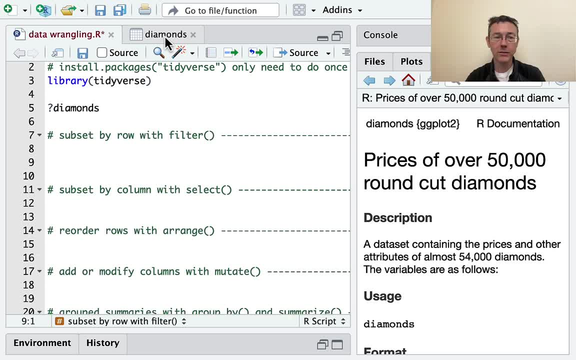 So let's jump in with filter. Let's subset by rows. So, looking at the diamonds data set, maybe I just want the ideal cut diamonds. So let's start with that. I want to do a filter and the first argument is going to be the name of the data set. That's going to be a. 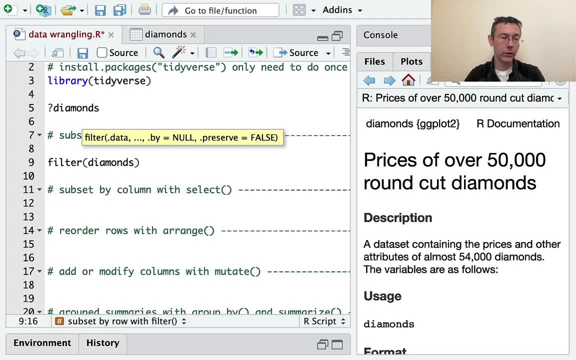 trend in all of our data sets. So let's go ahead and do that. So I'm going to go ahead and select all of the verbs I'm going to be using today. All of these functions take as their first argument the name of the data set And, as we'll see later, this is very 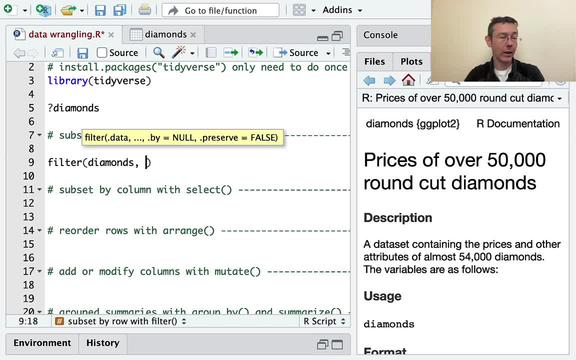 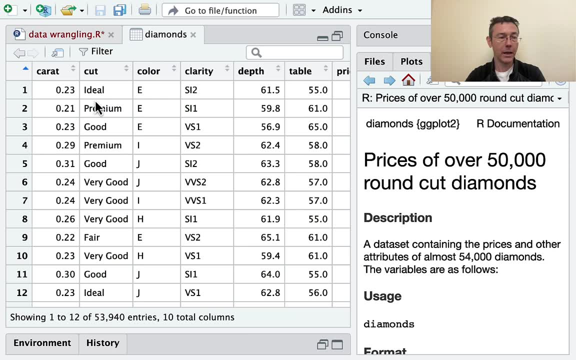 convenient in a lot of ways. After that, we need to say what we want to do. What's our criteria for filtering, And in this case, my criteria is going to have to do with the cut column, And I want to save only rows that have a certain value of cut The way I denote. 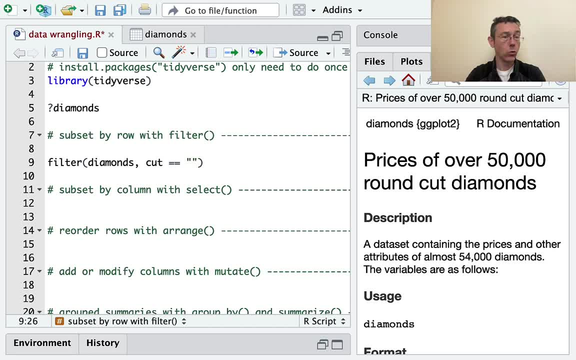 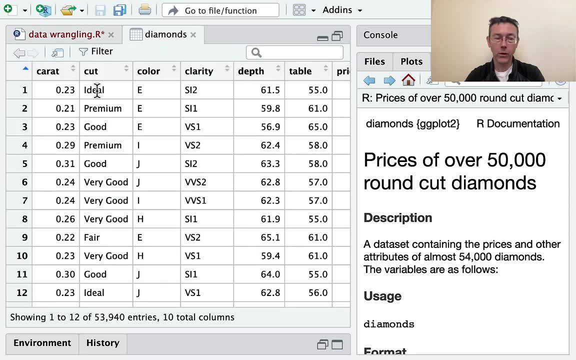 that is cut double equal sign and then in quotes the thing I want. So in this case it's ideal. I'm going to put it in quotes here because this is a string, It's just characters, right? So I need to let R know that I'm not talking about a variable called ideal. I actually 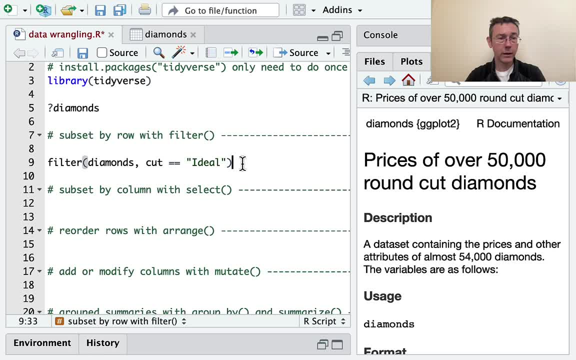 want the values. ideal Now, if I print this out, if I hit enter right now, if I execute this, it's going to print out in my console. It's going to be ugly. I don't really want that. I'm going to rename this as diamonds- How about diamonds small? And I'll command. 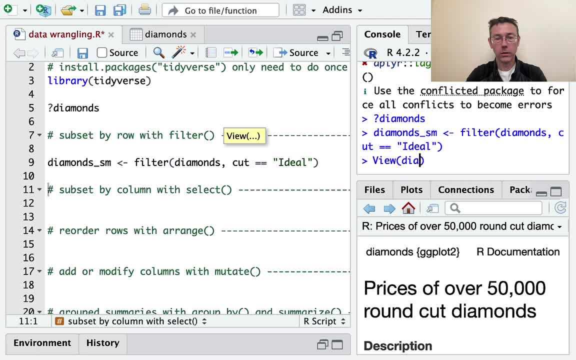 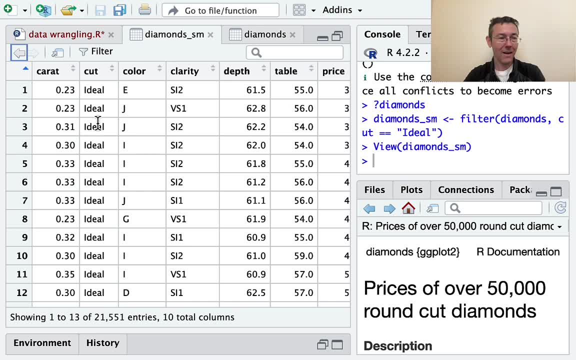 enter to execute that. And maybe I'll put that in my viewer: Diamonds small. And I'll put that in my viewer Diamonds small. And I'll put that in my viewer: Diamonds small. I'm going to mistype a lot in this vid. I'm sure I'm sorry for that. All right, So there. 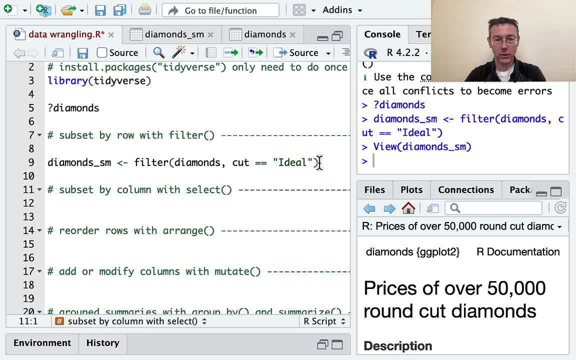 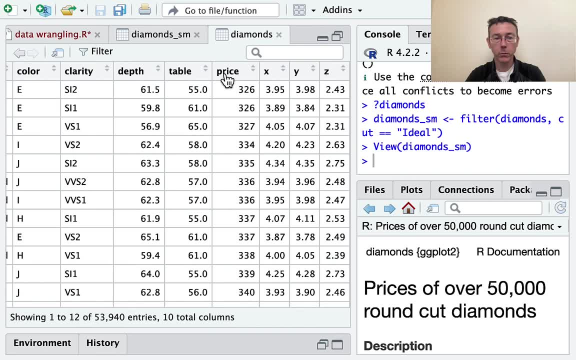 we go, You can see we only have ideal cut diamonds. Great, What else might we want to do? Well, we might want to subset by a quantitative variable, For instance, let's just take more expensive diamonds. We've got price here, So again diamonds, small, Maybe I'll just 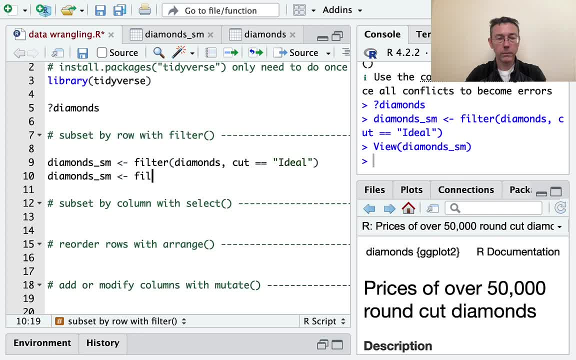 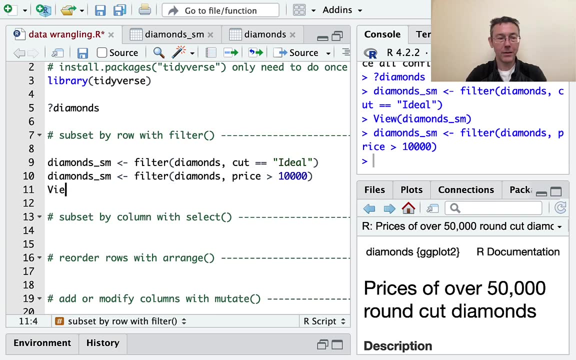 copy and paste that. I'm going to do another filter Again. diamonds is the data set I'm working with And my criteria now is going to be based on price. I want things that are over $10,000.. So those are going to be my more expensive diamonds. Maybe I'll put that. 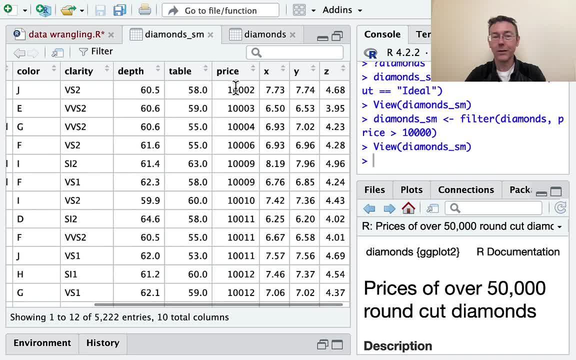 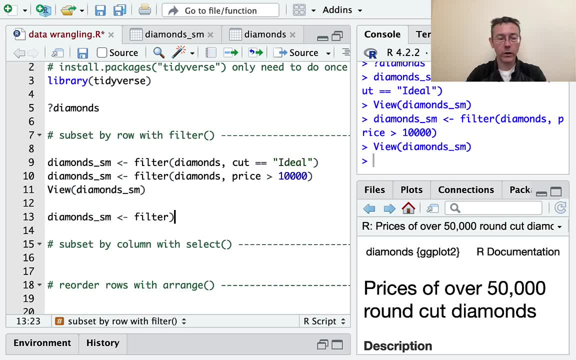 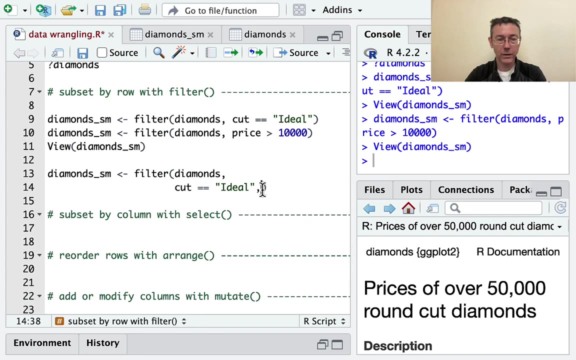 in the viewer. So now you can see only ones with big prices. We can do multiple criteria. So let's see here, Let's take a filter on diamonds And let's do both of these things. And since I'm getting multiple arguments, maybe I'll do this vertically, just for legibility. 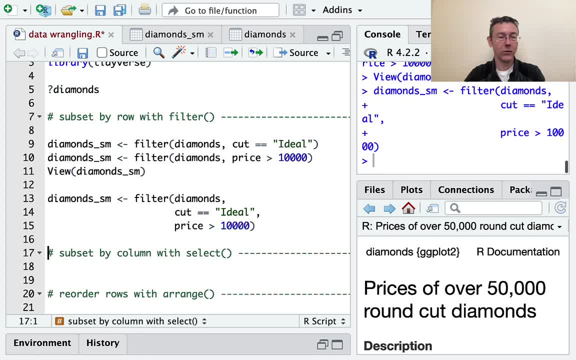 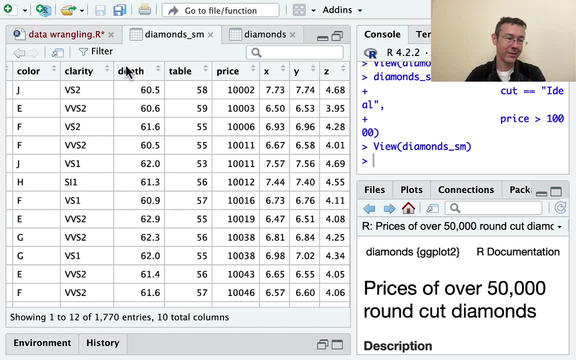 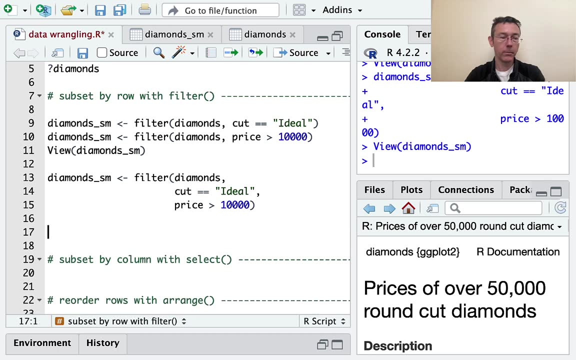 Let's also take price greater than $10,000 and see what we get. We can view that again. All of these are ideal cut diamonds. All of them have price over $10,000.. So you can see, just adding a comma here allows you to do sort of an and when you're doing a filter. 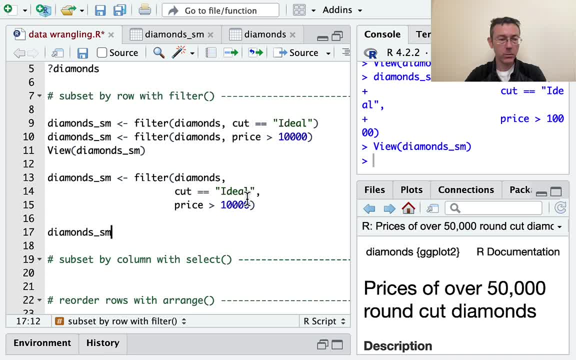 To do an or, the syntax is slightly different. Let's do that. You know, maybe I'll just copy and paste this whole line here, since it's pretty similar. If I want an or instead of a comma, it's a vertical bar, And so this: 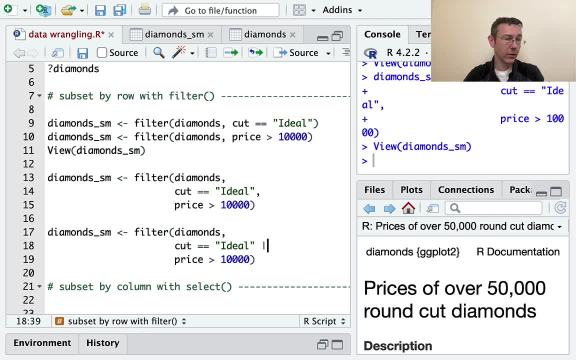 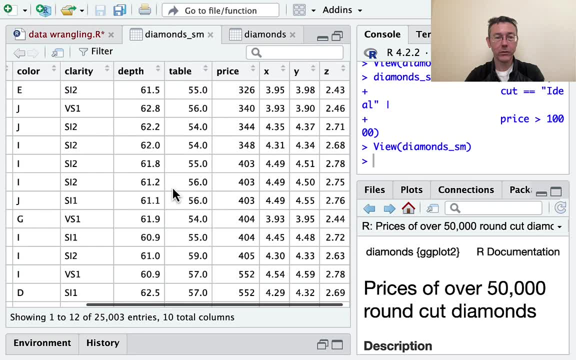 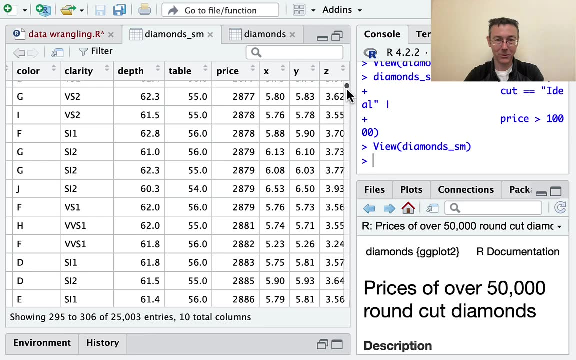 is going to give me all the diamonds that are ideal or over $10,000 or both. So it's not an exclusive or So ideal cut diamonds that are under $10,000.. And if we go further on in here, somewhere down here, there'll be some diamonds that are over 10,000.. I don't. 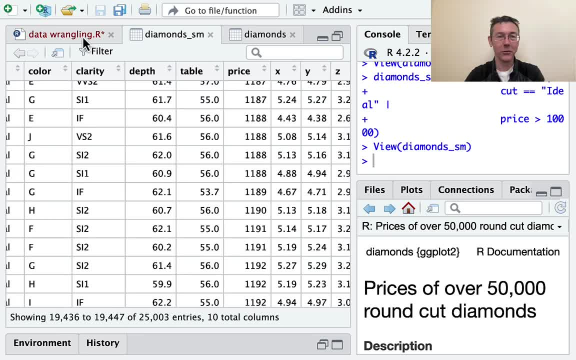 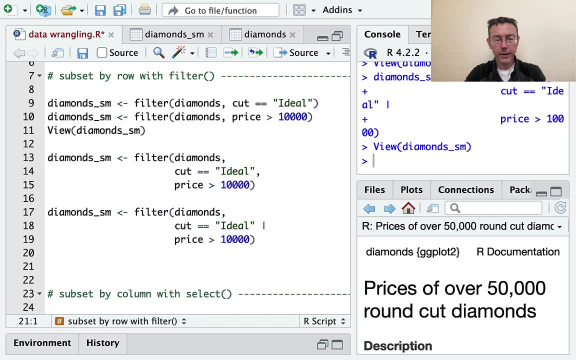 want to spend too much time searching, So I won't search at all. OK, So there's a lot of different things we could do with the filter. One other thing that I'll mention- I'm not going to do examples with this, but let's just mention it- Filter. 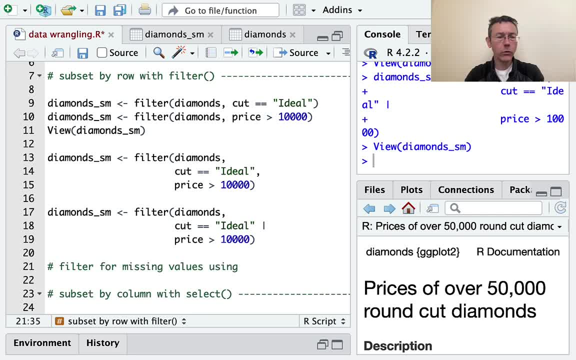 for missing values. You can't just do like cut equals, quote NA. That'll look for a character vector called NA. So you need to search for missing values using is dot NA And if you want aren't missing, you want exclamation point which is: there is dot na. so that's the not are things. 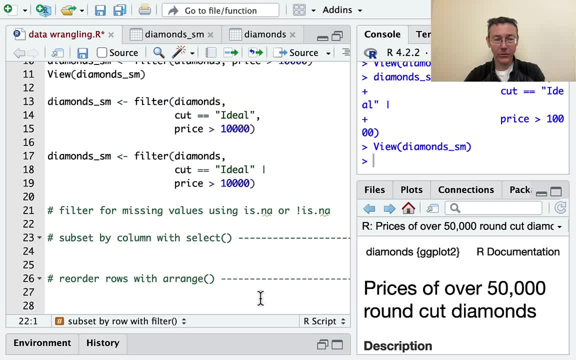 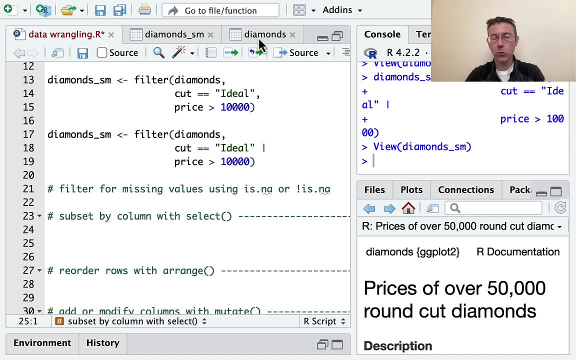 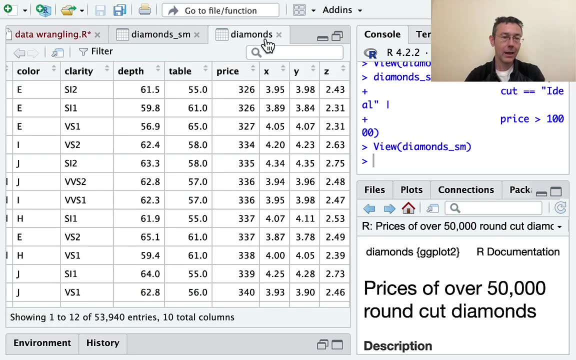 missing or are they not missing? all right, for the sake of time, i'm going to move on to select, which is going to let us choose columns within our data set. so maybe you've got a very wide data set, maybe it's got 100, 200, 1000 variables, 100, 200, 500 columns, and you don't want all of them for. 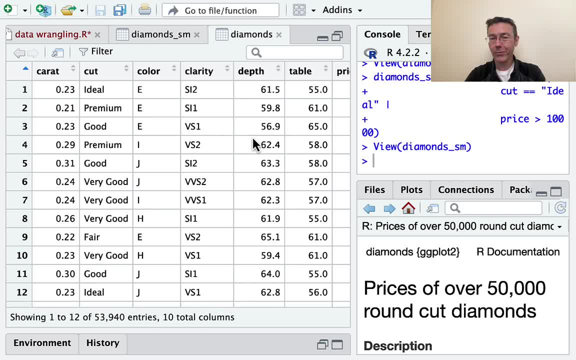 various reasons this might come up. so, um, the select verb is going to help you with that. it's going to let you subset columns. you can also reorder them and, if you want, you can use it to rename your columns. so, for instance, let's let diamonds small. i don't need all of that. 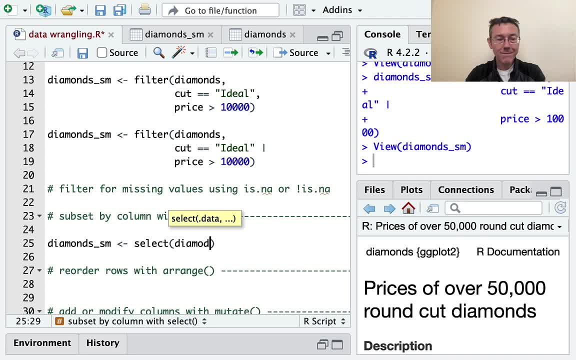 uh, be selected from diamonds and? um, let's just take cut and color, let's make it really small. so you're going to want to make sure that we have a lot of space, so let's make sure that we have. let's make sure that we have a lot of space, so let's make sure that we have a lot of space. so 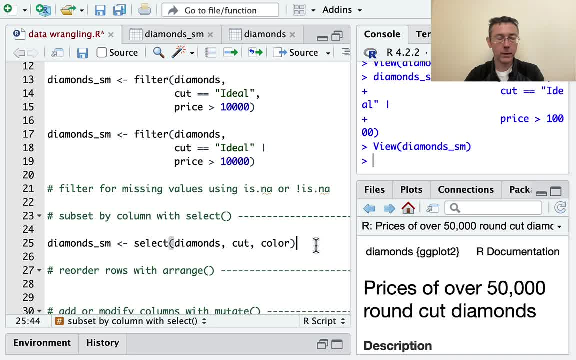 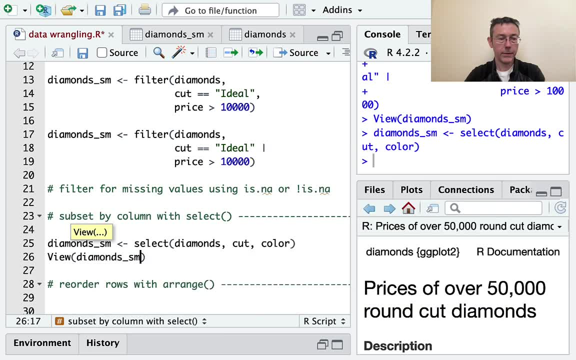 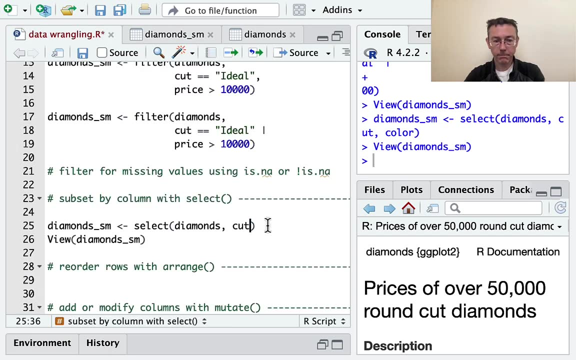 you know, say i'm using comma here again as sort of an and statement. if i do that and then view diamond small, you can see i've just got those two columns, just the ones i named. if i reverse the order color before cut, it reverses the order here too. now you can specify the columns you want in. 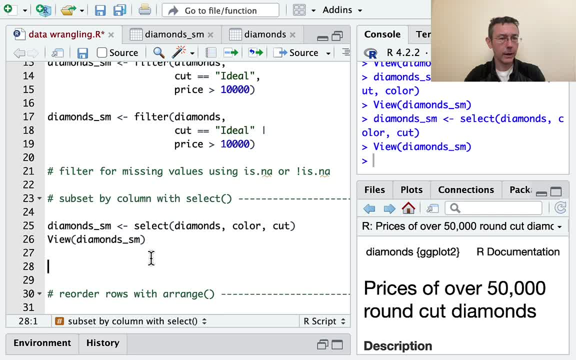 many, many, many different ways. the name for the general vocabulary for picking columns in tidyverse is tidy select syntax. i'm going to teach you just a little bit of that. so, um oops, let's take diamonds small again, and this time we'll do a select on diamonds, let's just do the columns. 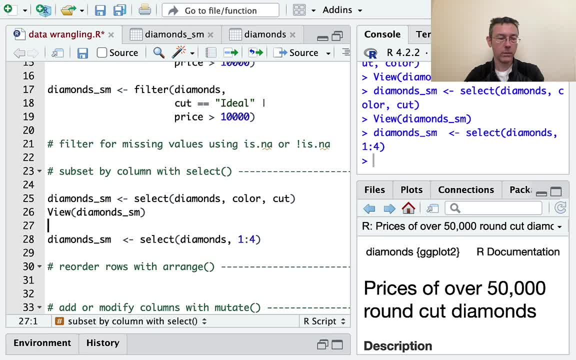 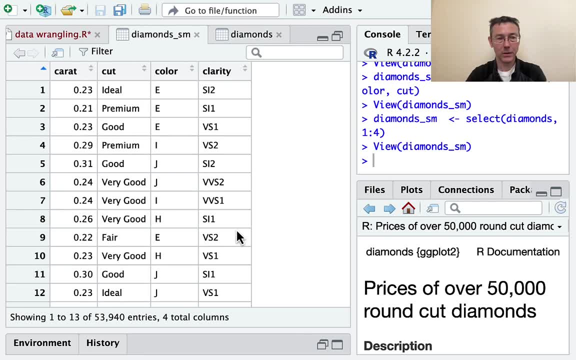 that we want by number. so let's just take columns one to four. you can see we got the first four columns of diamonds. you can see we got the first four columns of diamonds. and then we're going to do the columns carrot, cut, color and clarity. so you can do them by name, you can do them by number. there are a lot. 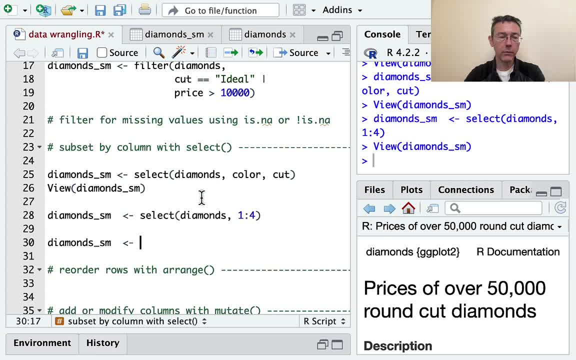 of helper verbs, just sort of little smaller verbs that give you- um, well, they give you a little help with your select. so let me show you one of those. so in the diamonds data set, let's just get all the things that start that start with c. so instead of having to list out, cut color clarity, etc. 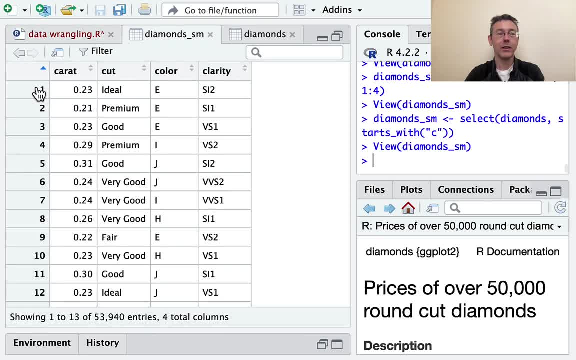 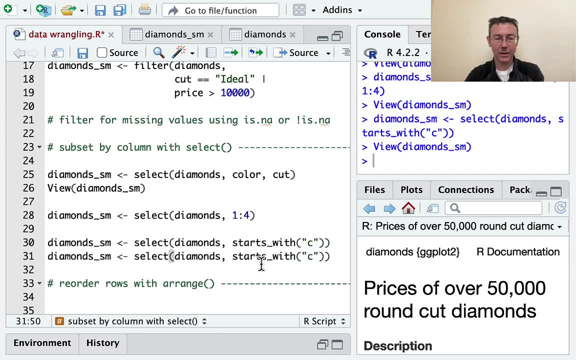 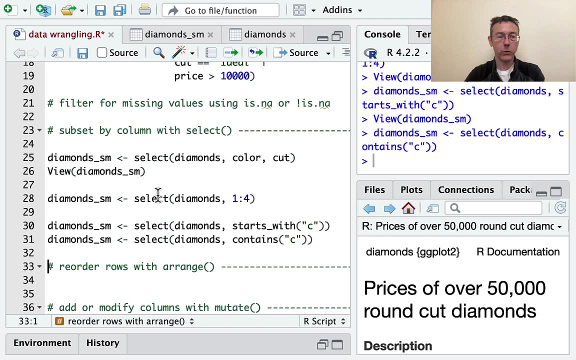 this is just going to. let me pick anything that starts with c. you can see that there are four such columns. i'll copy and paste that to show you one more like that. there's also ends with, by the way, another one that you might want is contains, and so contains is going to get the four that we. 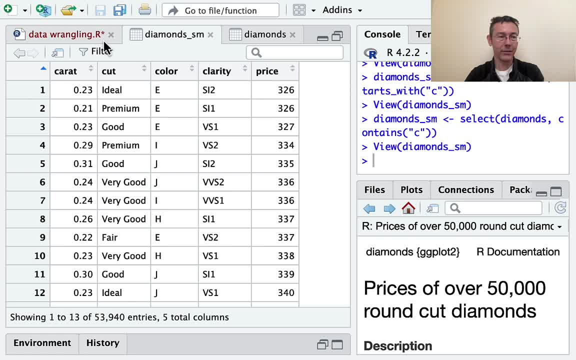 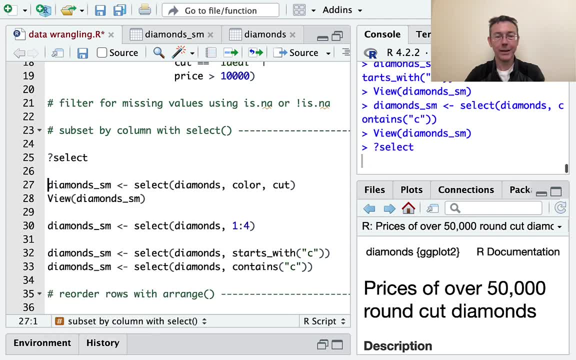 had plus price. those are the only columns in here that have a c. uh, you can learn a lot more by the way about this. i'll put this up top with question marks and then i'm going to go ahead and do a question mark select, get you the whole help file on that. lots of help there. let's go up and remind. 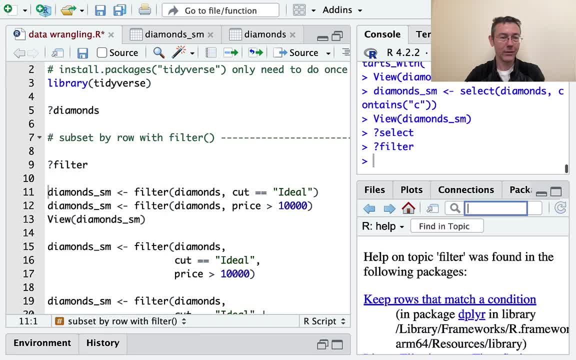 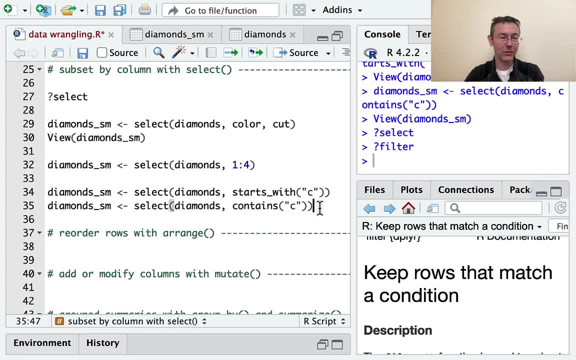 uh, and put a note in here that you can also do question mark filter. i think that's useful and it's the one from the dplyr package. so obviously in this vid i'm not going to get to everything, but this is some helpful stuff. one last one i'll do with select. oops, i don't want. 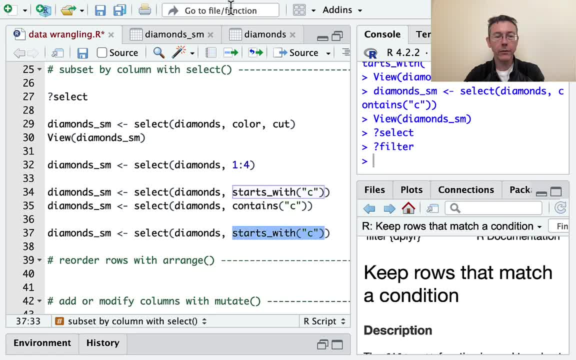 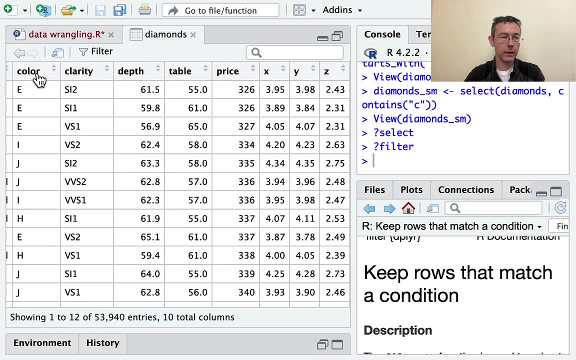 starts with c. uh, let's just say that we have the diamonds data set and let's say: i just want to put price up front. well, i could put price and then put all of the other ones, for instance, you know price, then cut, etc. but there's a helper verb for this too, and that's everything. 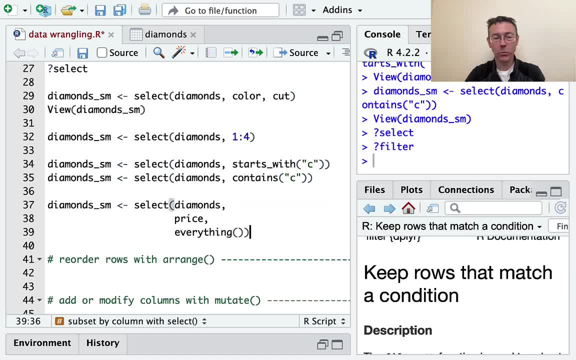 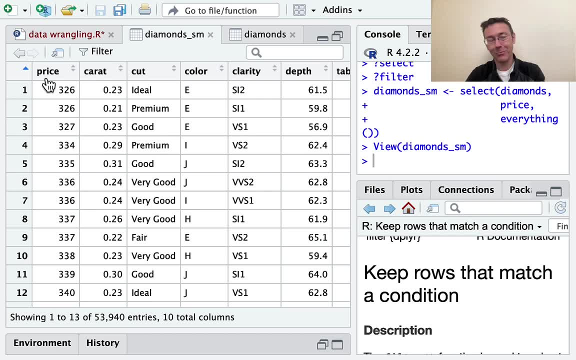 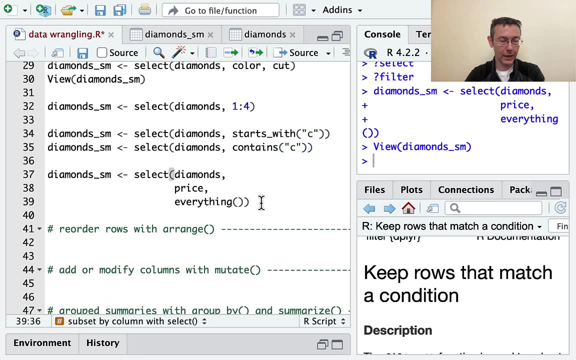 which i do have to type correctly, and this is a function, so it gets parentheses after open and closed, and if i do this, you'll see it's the same data set, but it's got price up front, just like we want, all right, so, um, this is once again a really deep well, there's a whole lot. 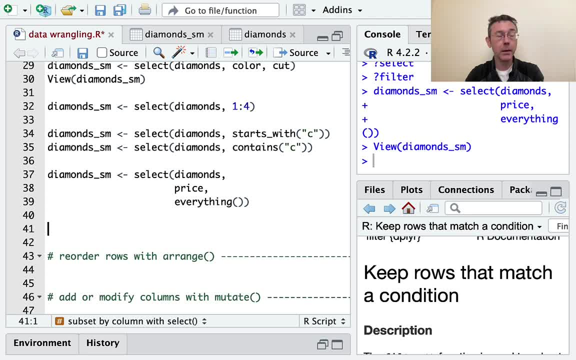 oh, i do want to show one more thing, like suppose we just wanted to eliminate one row, i'm sorry, eliminate one column. so this time i'll take diamonds. let's just take out price and you'll see, i did that with a negative sign, so this is going to give me all the columns. 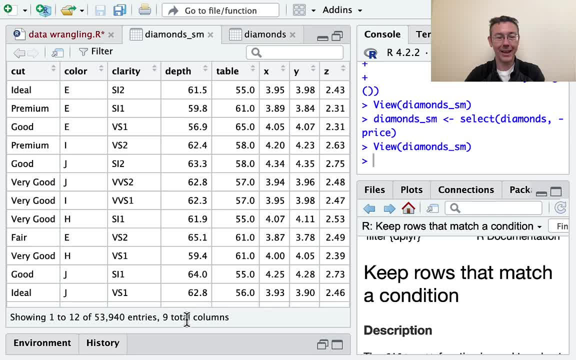 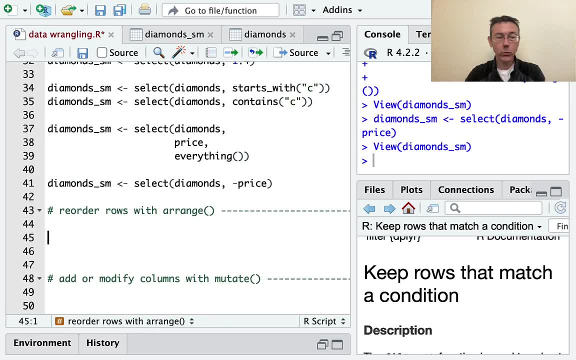 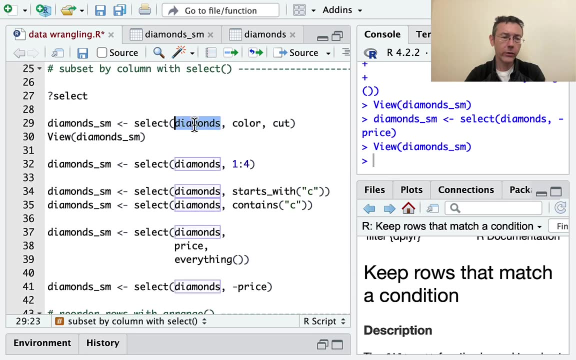 except for price. this new data set only has nine columns instead of the original ten. price has been removed. okay, let's reorder some columns with a range. now, as we get into this, you see that we're always having the data set as the first argument. also, when you're doing real world data analysis, you'll 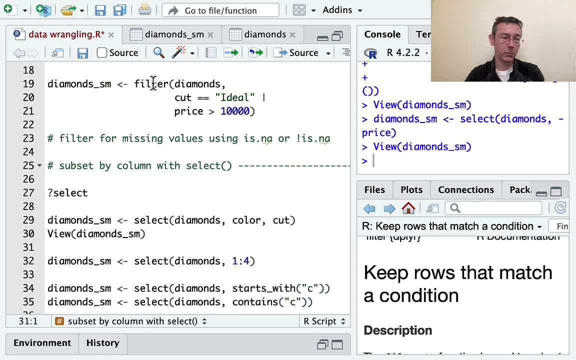 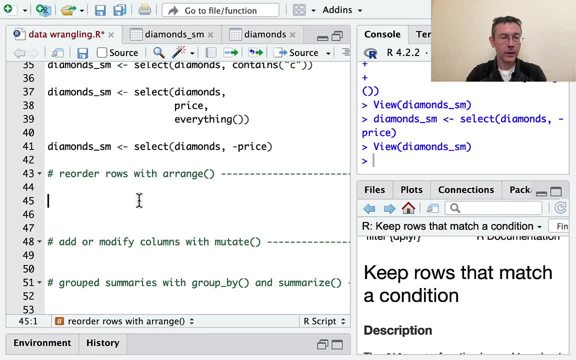 frequently want to do each of these things. you might want to do a filter by row and then only select some columns, then reorder them. you end up with a whole data analysis pipeline, and so tidyverse r is set up for this, and so i'm going to just rewrite some of this. 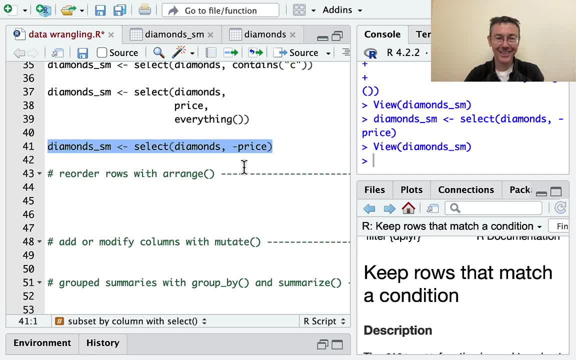 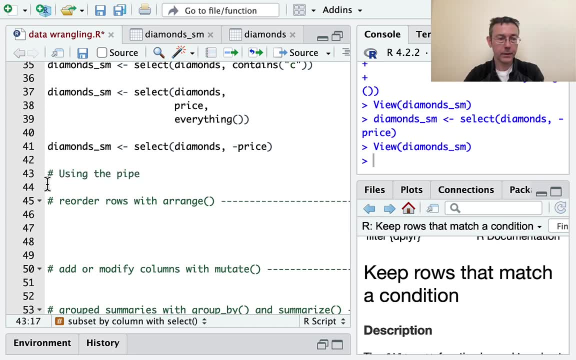 a little bit different. let's just: i'm getting to a range. i promise let's just rewrite this in a different way and i'll comment it. i'm going to use the pipe and it's going to bother me if i keep that capitalized. so the pipe is going to be exactly the same thing as this, but it lets us. 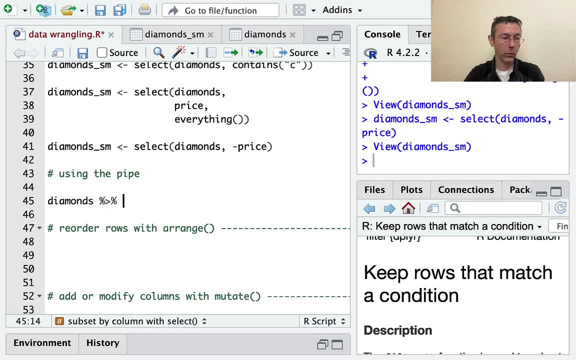 write in subject, verb, object order. so the subject of my sentence is diamonds. the thing i want to do is to select. and what do i want to select? i want to take out price, prints, price and again i want to save it as diamonds small, so i'll put that in here. 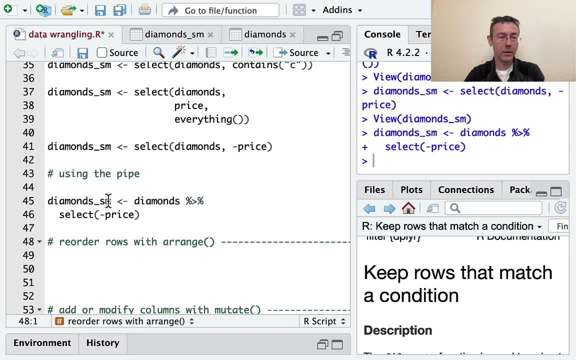 okay, that's going to be exactly the same. notice that what's happening here is it's taking the diamonds data set and passing it using this pipe as the first argument to the select command. this gets really helpful because all the dplyr verbs have a data set as their first argument and they 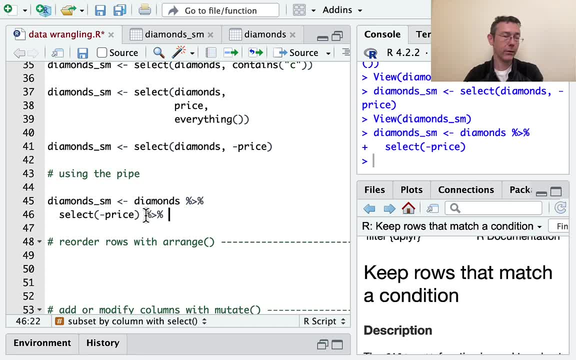 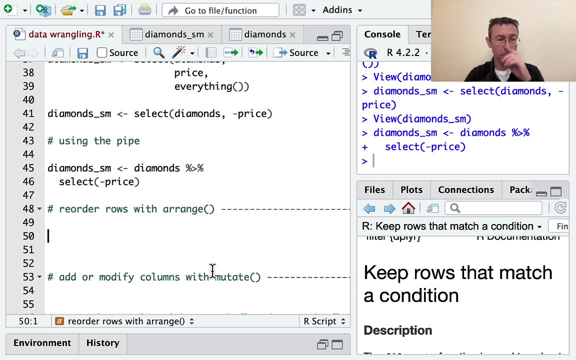 also output a data set. so if i wanted to put another pipe in here with, for instance, a filter, i could. by the way, the keyboard shortcut for this pipe is command shift m. i use that shortcut probably more than any other command, any other shortcut in r, so maybe in a little bit i'll do. 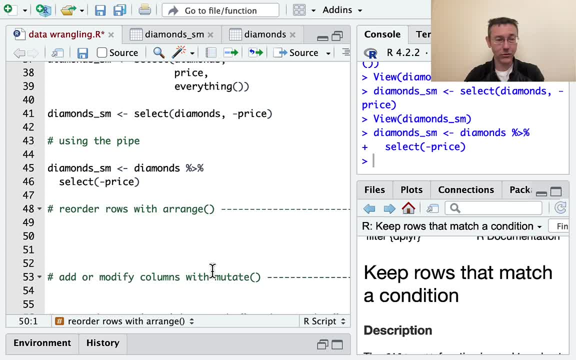 an example where i do a filter and a select and arrange and other things. you'll definitely see a longer pipeline where that gets useful. okay, so a range, lets us well arrange the columns, that, i'm sorry, arrange the rows that we have in different order. so, for instance, maybe 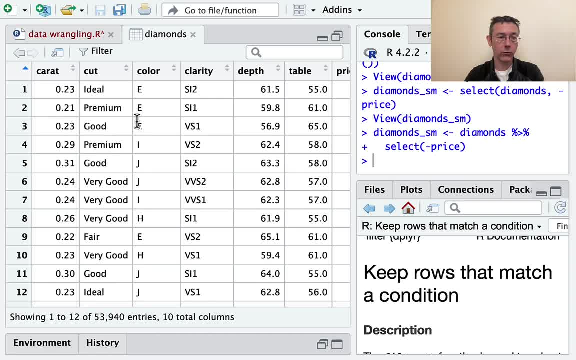 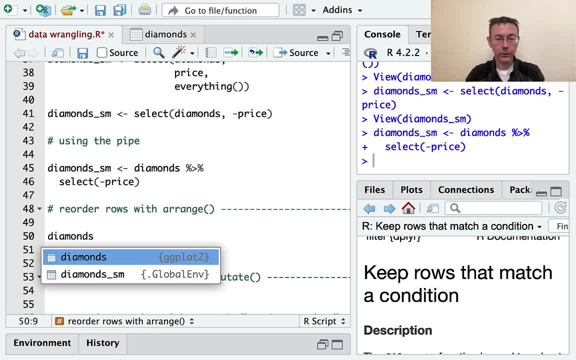 i want the colors to be in order. right now they're all kind of jumbled up, or maybe i want the carrots from small to large. so, uh, let's make a new name for this: diamonds, arr for arranged, and i'm going to start using the pipe, i'm going to take diamonds and then i'm going to arrange it. 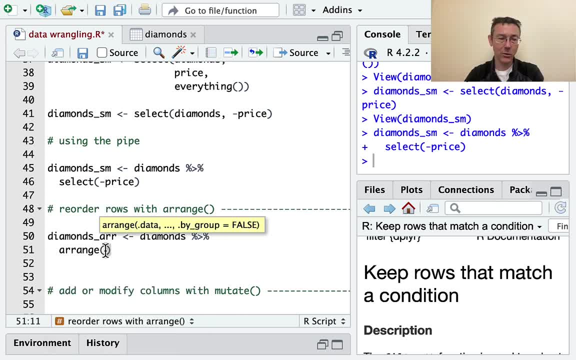 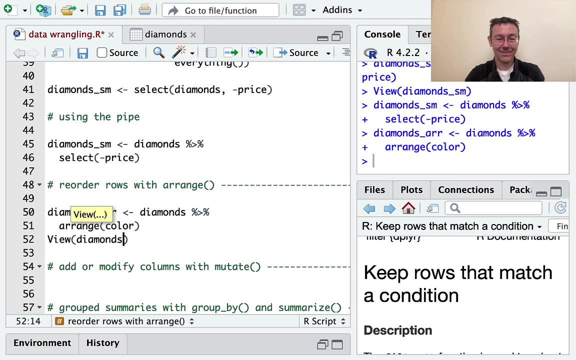 and here the way i'm reading that take diamonds and then arrange it by whatever criteria. so really, all i need to do is specify the criteria. let's, let's arrange it by color to start with, and we can view that. there we go and you can see color d and then, if we go further down, we'll have color e. 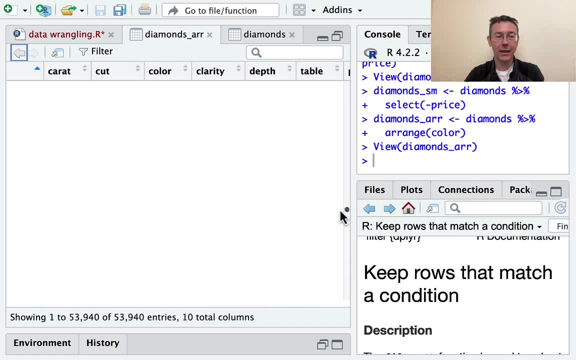 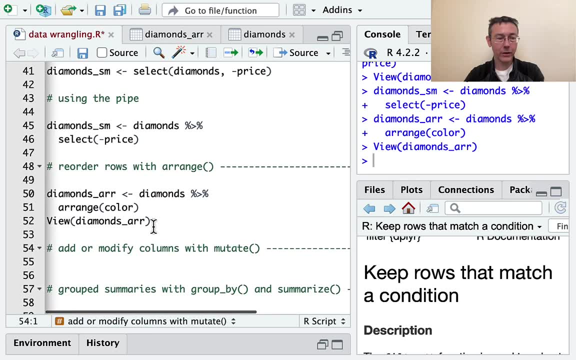 f, g, h. so it's going alphabetically in a written ascending order, sort of from a to z. uh, let's see here. i'll just copy and paste for a second, because i'm not going to be changing a whole lot this time. i'm going to arrange it by a carrot. 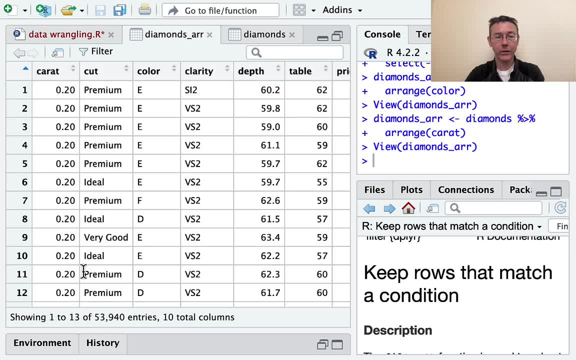 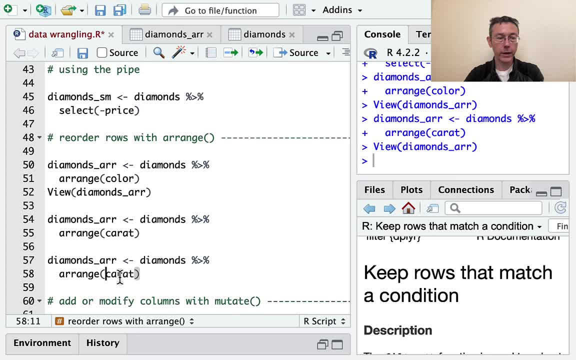 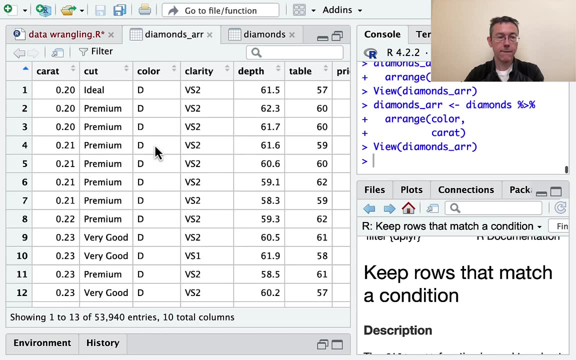 and you can guess what that'll do. ascending carrots. you can arrange by multiple things, sort of in order. so i'm going to arrange first by color and then by carrot. so all the d's are first starting with the lowest carrots, but i stick with d as the carrot gets larger. now we can reverse that order. 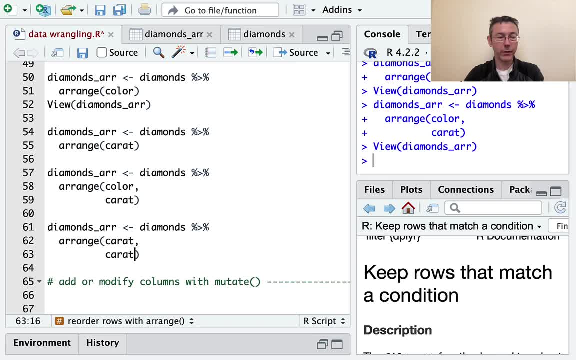 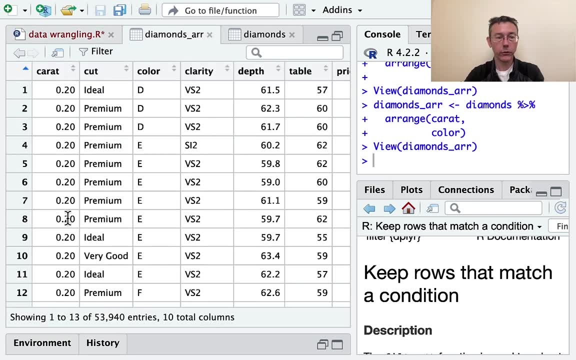 and get the columns arranged in a different way. so first let's arrange by carrot and then by color, so the smallest are first, but among the 0.2 karat diamonds, first we've got the d's, then the e's and so on, and you can arrange by two, three, four, five criteria, however many you like. um, i think that's. 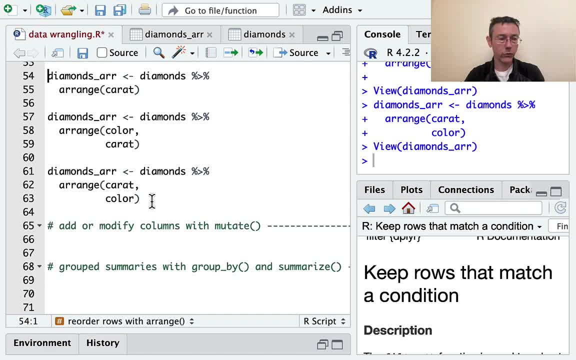 really all i want to do. oh wait, no, there is one more thing i want to do with the range, because you might not just want the smallest carat diamonds up front, you might want the biggest up front. so there's a couple ways to do that. the first is to wrap the thing in desc for descending. 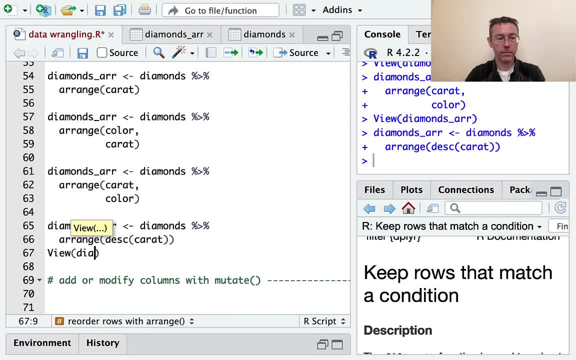 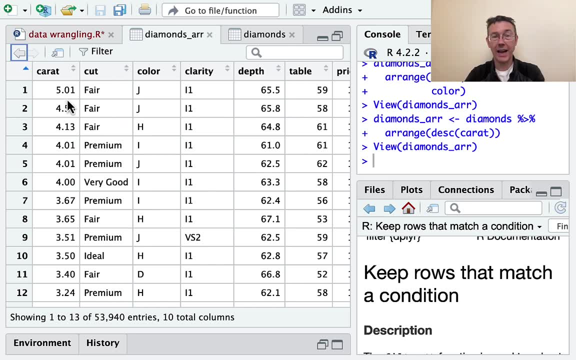 and let's view that there we go, okay. so now the biggest diamonds are first. so we've got this five carat diamond. that's a pretty big diamond. it's only got a fair cut, though, and then the numbers get smaller and smaller. one other way that you could do that, by the way, is instead of desc, you can put a negative. 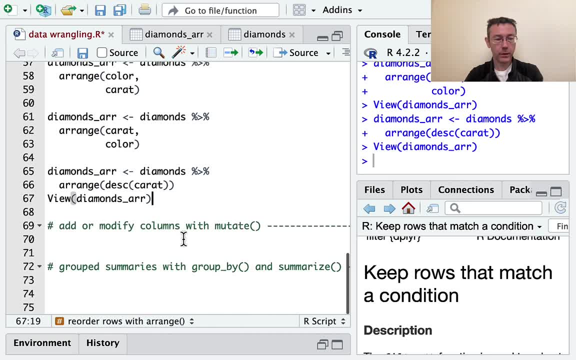 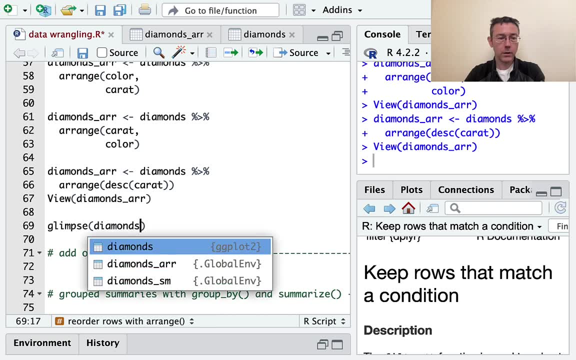 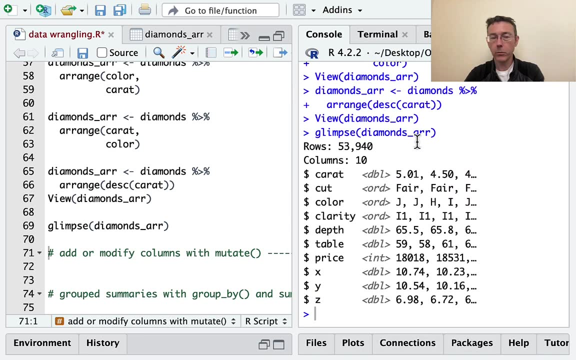 sign in caret. that ends up being exactly equivalent uh. before i move on, let me just show you one other smaller d player verb, and that's glimpse. so let's do glimpse of diamonds arranged and you can see that puts uh. it makes it print out in a way. 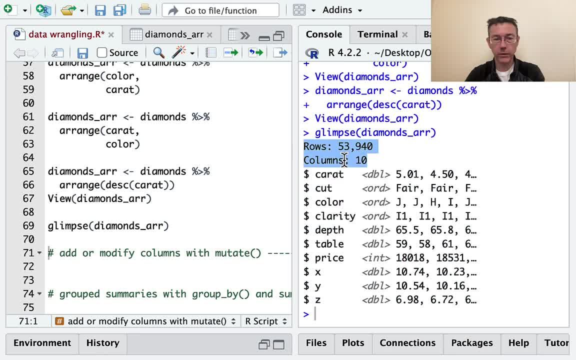 that's a little bit more legible sometimes fits in a little better. with a markdown document, for instance, you can see the number of rows, the number of columns. you can see each of the variable names, it's type and the first few values. and the first few values are chosen so that they fit in with. 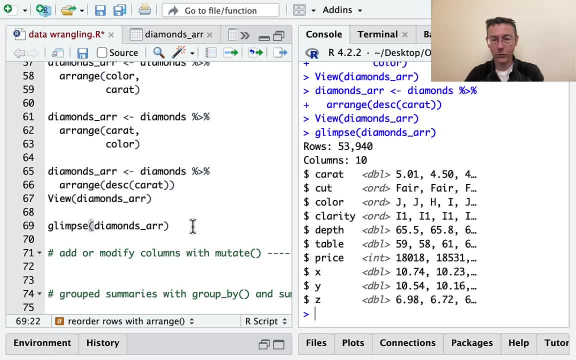 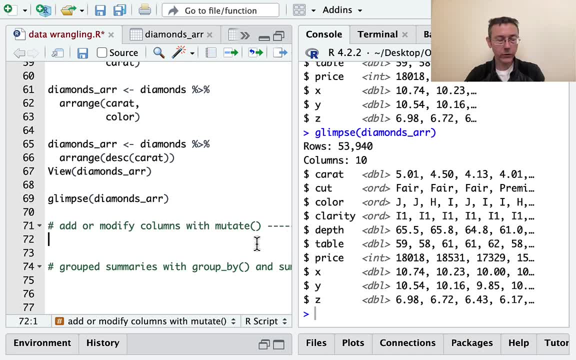 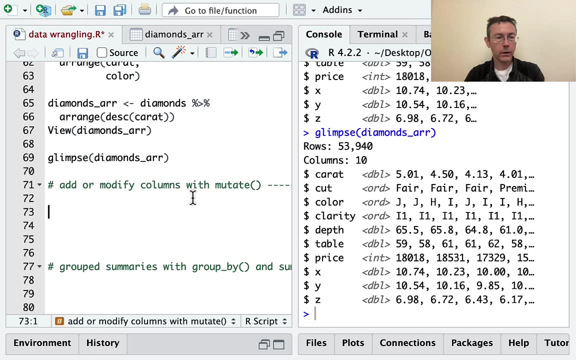 the console window. so if i rerun glimpse after i've resized the console window there i get a slightly different printout, i get slightly more values. so that's kind of nice, just a handy verb to have around in general. okay, let's modify and add columns with mutate. so there's lots of things. 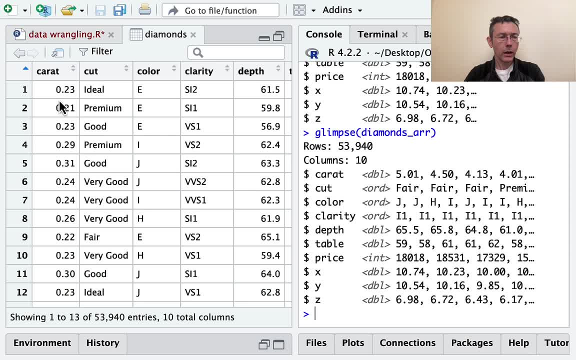 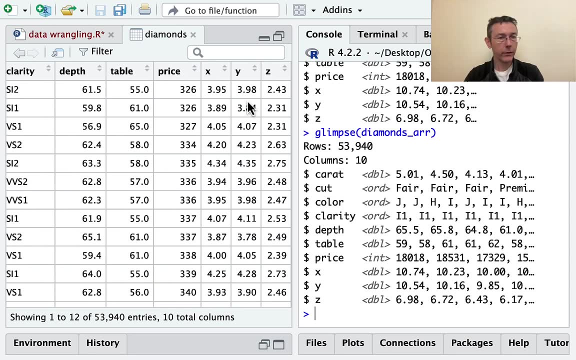 we might want to do here, clean up a little bit. uh, for instance, carrots are um a unit of measurement. that's wonderful for jewelers, but if you're like me, you don't necessarily have great intuition as to how much a carrot is, so maybe you want to add a column here that's going to convert carrots. 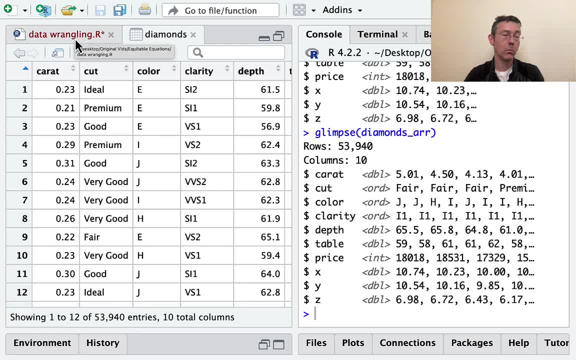 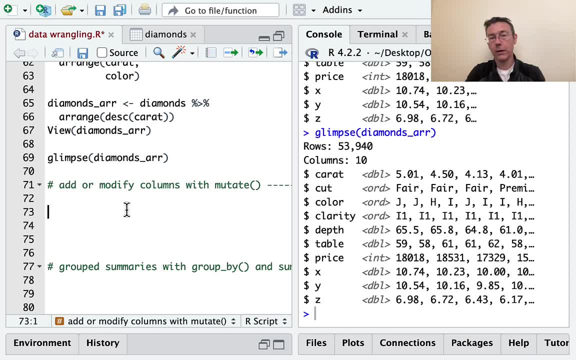 to say grams, and i happen to know, i happen to have looked up before, that a carrot is 0.2 grams. so let's make that modification and add a column to this data set with carat weight, with the mass of the diamonds in grams. so how about diamonds? uh, new, i don't know. 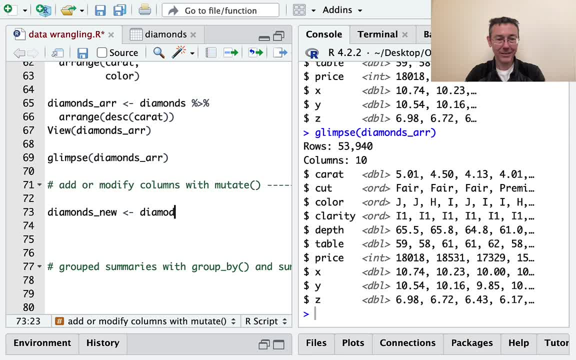 i'm not thinking too hard about my variable names today. i'm going to take diamonds and i'm going to pipe it into the mutate command. that's our new one. so again, diamonds now is passed as the first argument to the mutate commands. so take the data set and mutate it so that we have a new column. that's what mutate is going to do, and 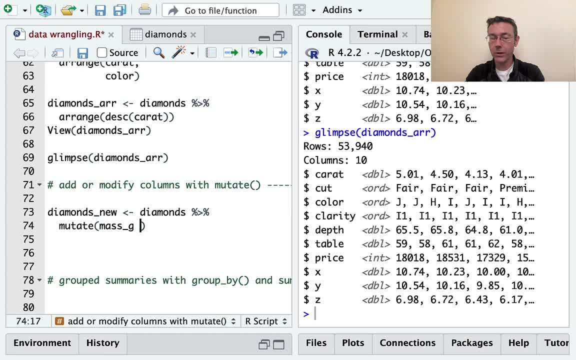 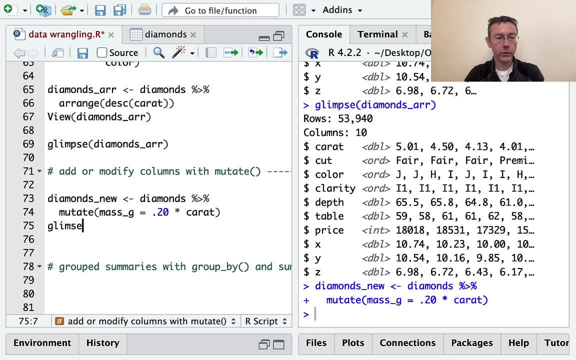 how about? mass g will be the name of our new column, and it's going to be defined to be 0.2- 0.20 times a carat, because each carat is 0.2 grams. and uh, let's just glimpse this. how about? 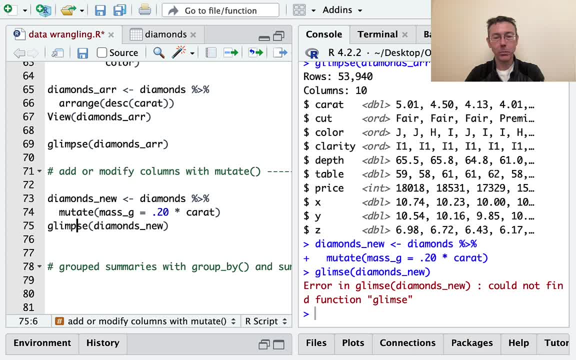 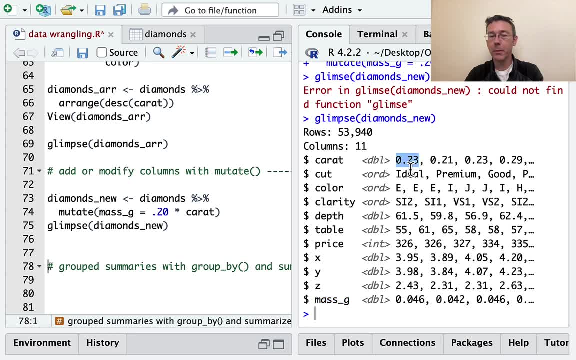 since we now have glimpse. yeah, r does want you to spell things right. i guess that's a good thing. you can see you've got mass in grams. so this 0.23 carat diamond has a mass of 0.046 grams. let's see here um a couple of the things we might want to do. 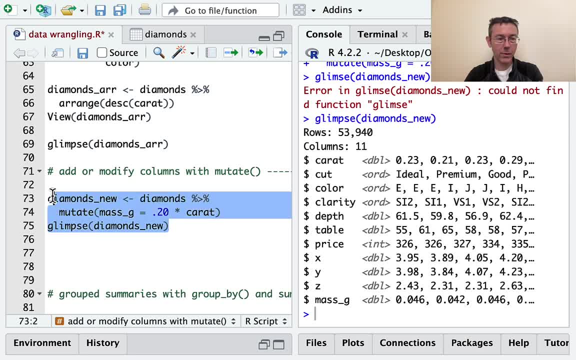 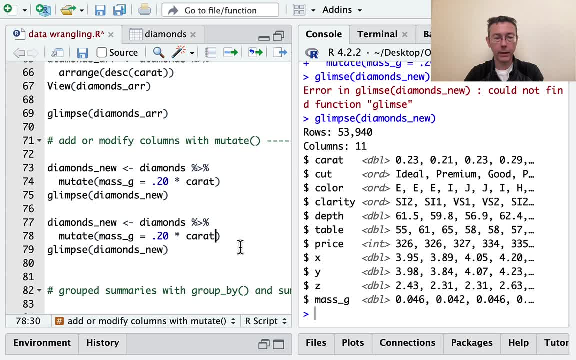 maybe i'll just copy and paste this whole thing, because i'll just stick with it and i'll add new things. you can add more than one column at a time. so um mass g equals: how about something like um price per carat? so what i'm going to do is i'm going to take price, and every row. 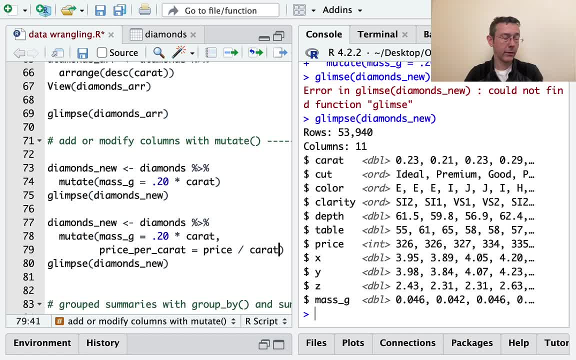 the value i get for price. i want to divide it by the value i get for carat. so these two vectors, mass g and carat- sorry, price and carat have the same length, and so r is just going to go through. compare component wise: 326 divided by 0.23. 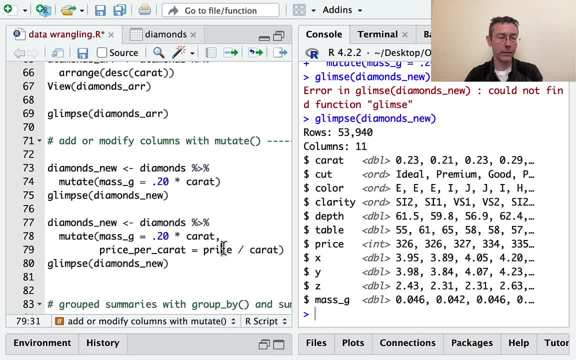 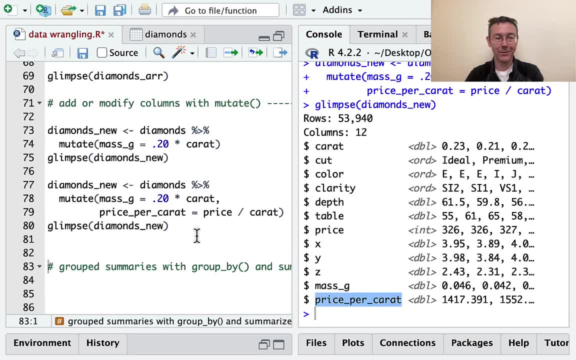 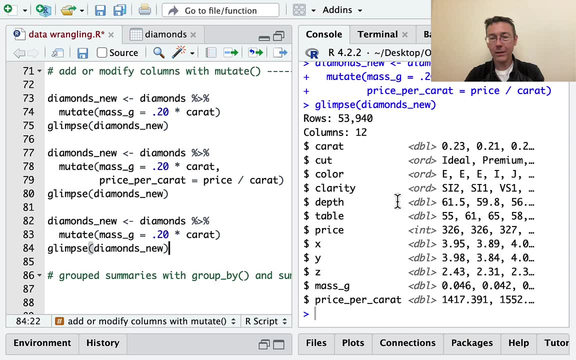 326 divided by 0.21, etc. and it's going to add a new column on that basis and if we glimpse it, you can see you've got your price per carat of your diamond. lovely copy and paste again. we can- uh, we can- modify column names while we're at it. so let's see here. you know what? 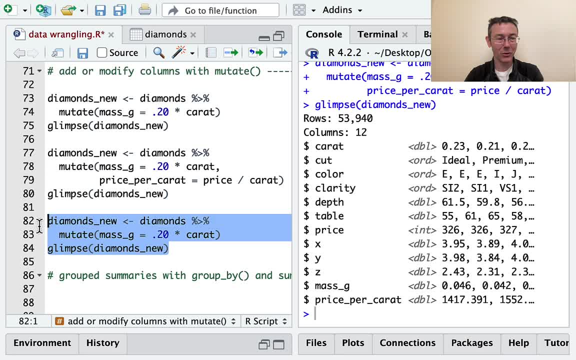 i think i actually want to copy and paste the larger set that i made. let's hold on to our price per carat one. let's modify the cut column, and i'm going to do it using an old-fashioned function to lower, and so what this is going to do is it's going to take all the values in the vector and make 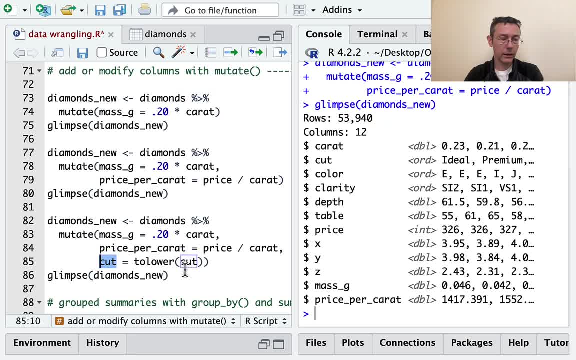 them lowercase. so notice i put cut equals. so r is going to see that that refers to an existing column and it's just going to overwrite it. so this can be useful sometimes. for instance, if i have no more use for these uppercased things, this would be good. 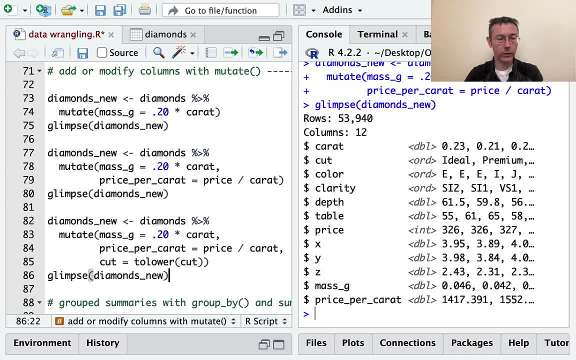 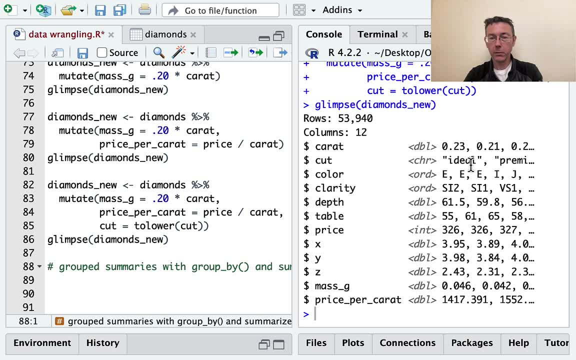 but it is kind of throwing away some information potentially. so there's not necessarily, uh, an easy way to get things back, depending on how your your workflow is going, and so if i do my glimpse, you can see that now my cuts are all lower case. let's see here. one last thing i want to show with mutate: 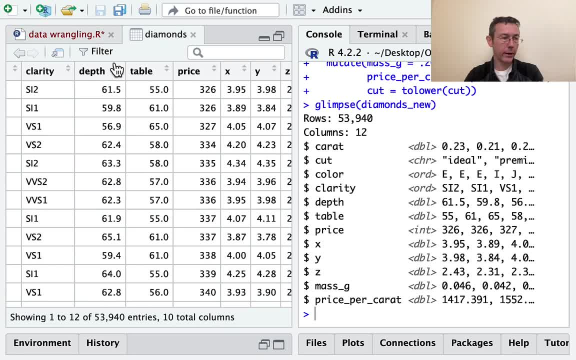 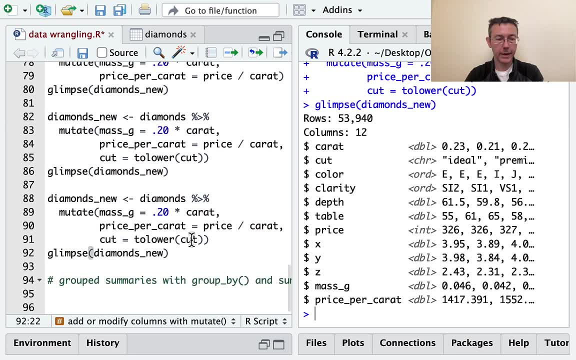 we talked about price right, and we filtered earlier for price being above a certain value. so i think i want to do one thing. i want to make a new column like that. so how about i make a column called expensive? how about yn for yes, no, or maybe like tf? i don't know. i don't want to think too. 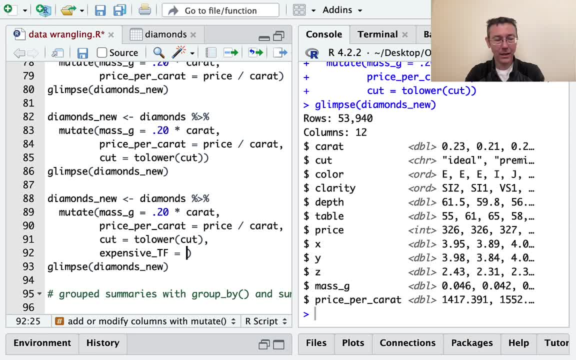 hard about my column names today. they're not always ideal, i know, so i'm just going to give it a logical condition. i'm going to say: let's call something expensive if the price is over ten thousand dollars. uh, for me expensive is much lower than that, but that's a different thing entirely. 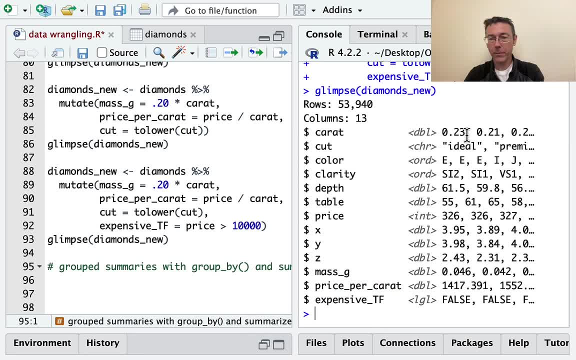 let's just take this on, uh as it's given, okay, so the price of 326 is not considered expensive. similarly, for these next few entries, this is a logical vector. it's all going to be trues and falses, great. so, um, that's all that i want to do with mutate. 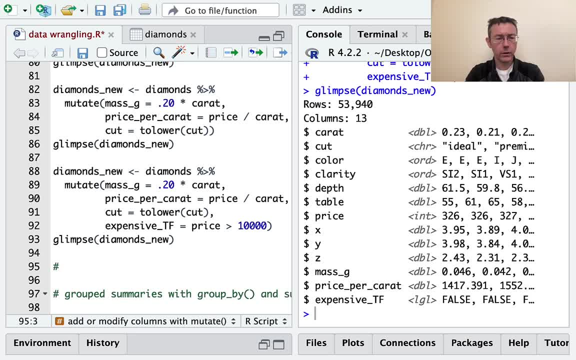 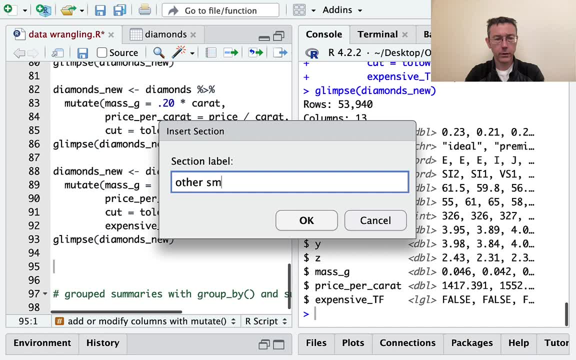 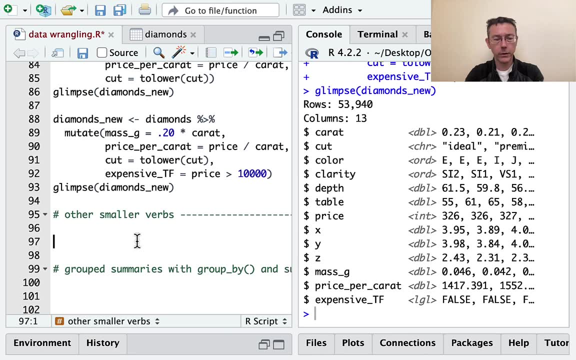 let's see. i want to to mention a couple others that are useful. Maybe I'll put a section in here. By the way, I'm getting a new section with command shift R. How about just other smaller verbs? This isn't going to be a complete list, but it'll be a few others that you might investigate on your own. 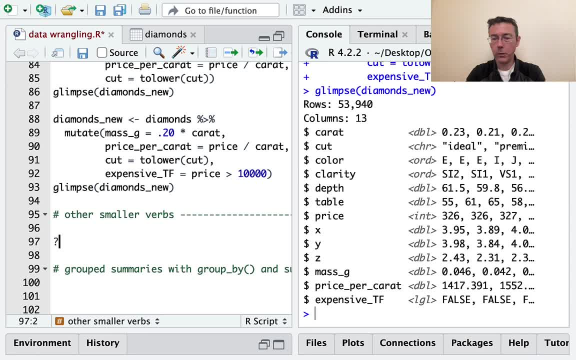 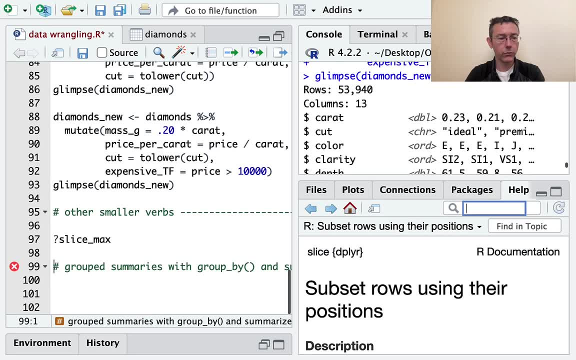 I'll do this as a comment. No, you know what. I'll do this for help files, So you might want to check out slice, like slice max and stuff. There's a few fundamental or there's a few functions in that family that are worth knowing: Subsetting rows using their position or other. 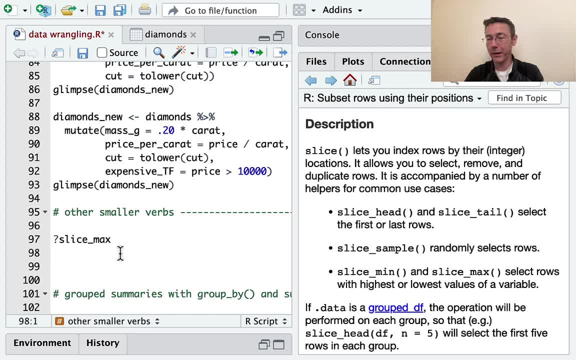 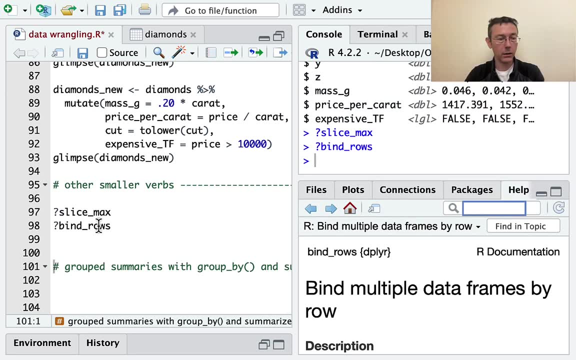 things. So this would subset by the biggest value of a variable or the biggest few values of a variable. I also recommend checking out bind rows. So this is where you have a couple data frames that are the same and that they have the same columns and you just want to latch them. 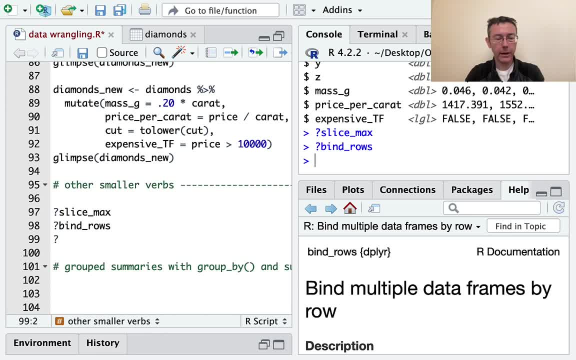 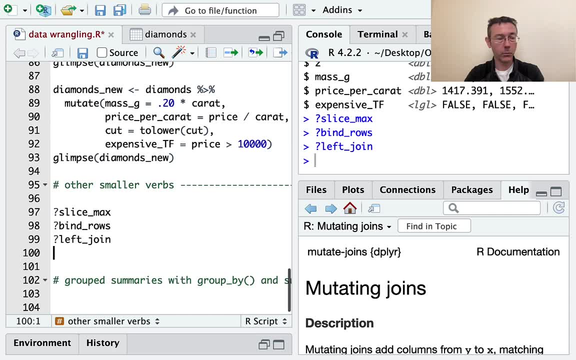 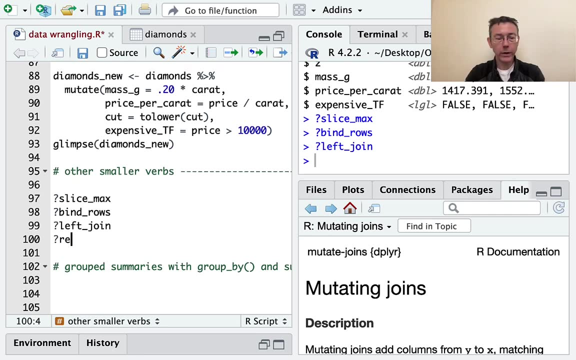 together. I am not going to talk about left join. Joining data sets that refer to similar information, the same observations, but may have different columns, can be really helpful. So check that out. Rename just to rename columns, That's a. 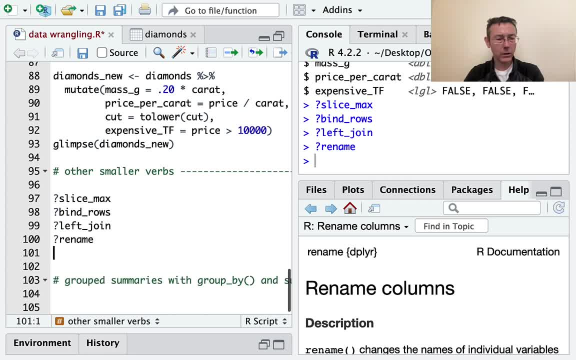 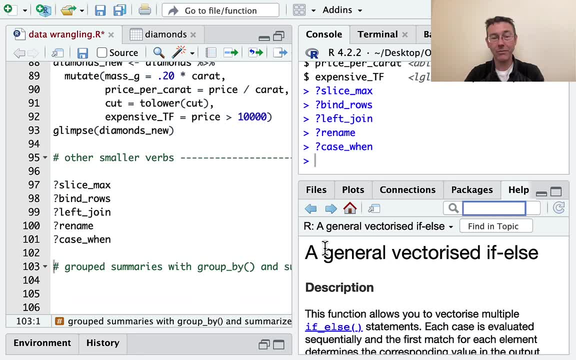 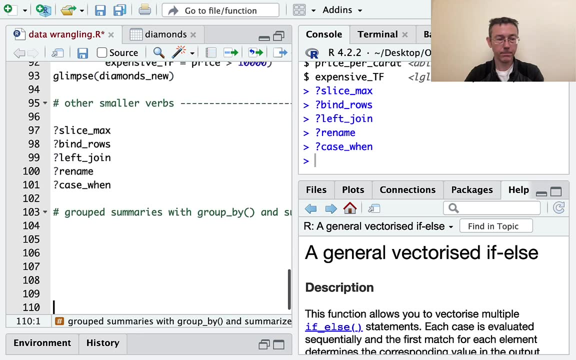 nice one, And I'll also mention case when- and I won't say anything really about that right now, but it's a generalized, vectorized if else, and that can be really useful inside of your mutate method, but it's definitely recommended. 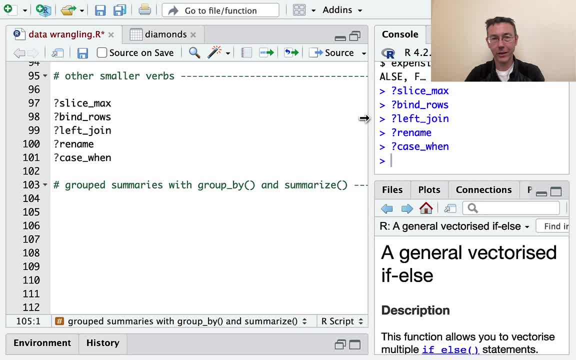 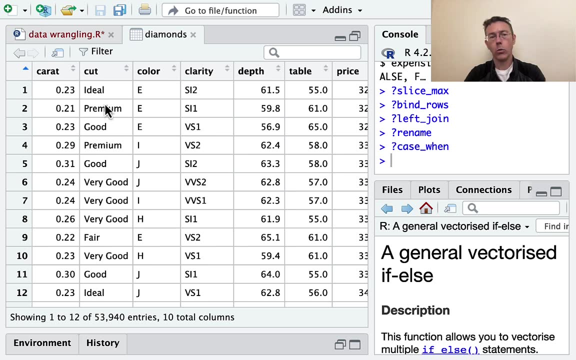 Okay, Grouped summaries. Someone once told me that all of data science, or 90% of data science, comes down to groups summarize, grouped summaries. It's an exaggeration, but not by too much. Here we're going to really see the power of the pipe. We're going to look at this diamonds data set and we're 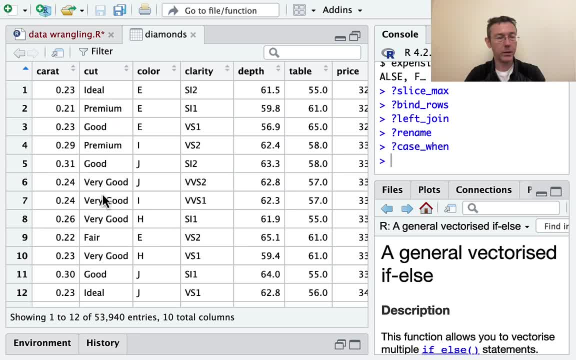 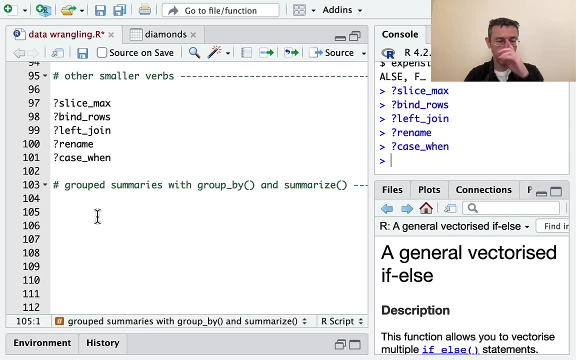 going to say, okay, what kind of caret weights are we seeing for the different cuts of diamonds or the different colors of diamonds, those ways? So what we're trying to do is to essentially group this data set by, say, cut or color, and then get some summary information on some other variable. I think the easiest way to 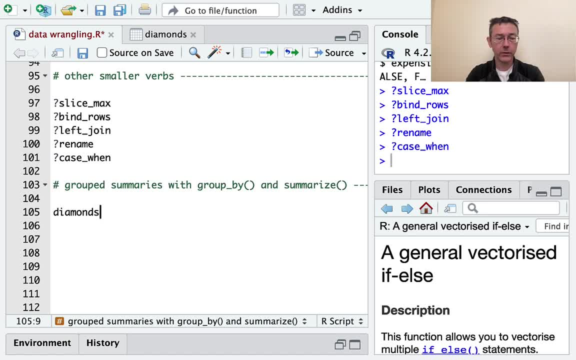 understand. this is just to dive in and do it. So let me do that. I'm going to take diamonds, I'm going to pipe it into group by And I want to group by. let's start with cut. And if I just hit enter there, not much is going to happen. I'll just print it out. 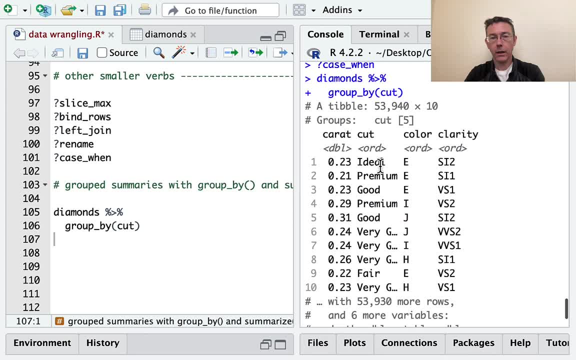 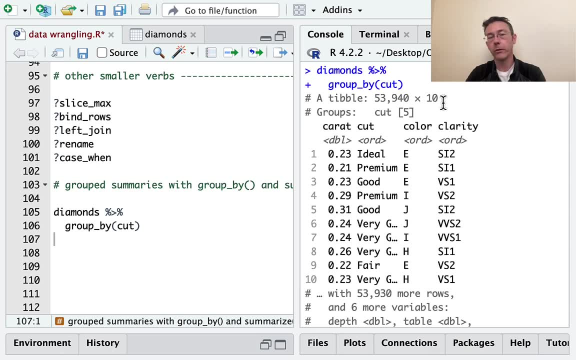 You don't really see the difference. I've still got the same data frame, the same tibble, Same data frames and tibbles are basically the same thing for most purposes. Underneath the hood tibbles are a little easier to work with. The only difference is that now this data frame 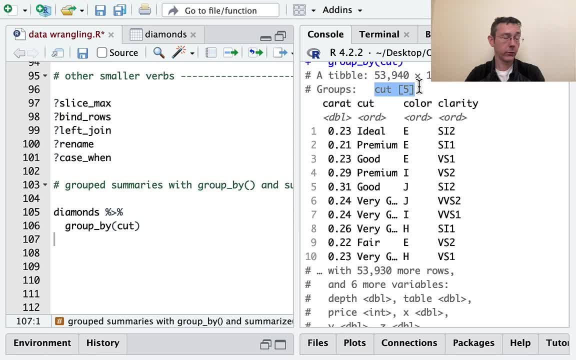 has a groups attribute- And I imagine this like if it were an Excel spreadsheet- that all the ideal cut diamonds are highlighted in one color, all the premium diamonds are highlighted in another. So then, when we're done with this, we're going to go ahead and do the same thing. 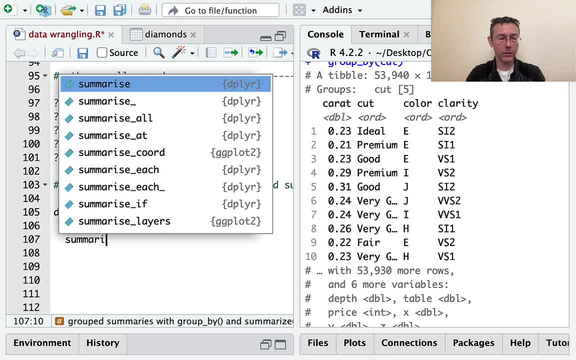 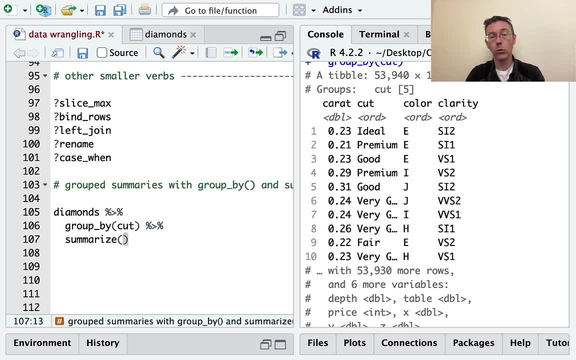 When I take that data set and put it in a summarize command like so: whatever command I give it, whatever summary data I ask for will happen. group wise. It'll be done for the ideal diamonds, the premium diamonds, the good diamonds, all separately. So, for instance, I can get the 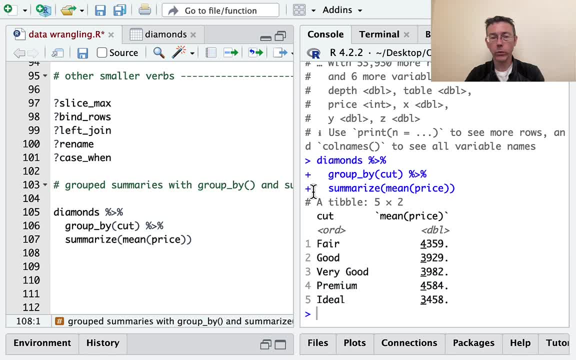 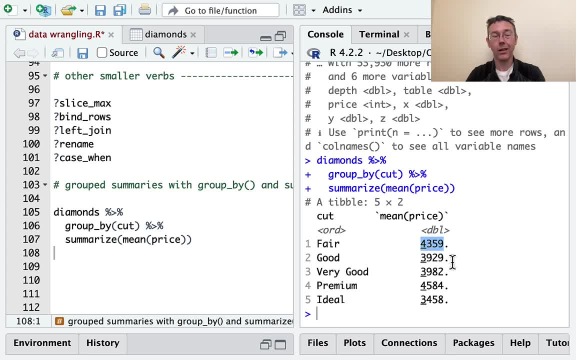 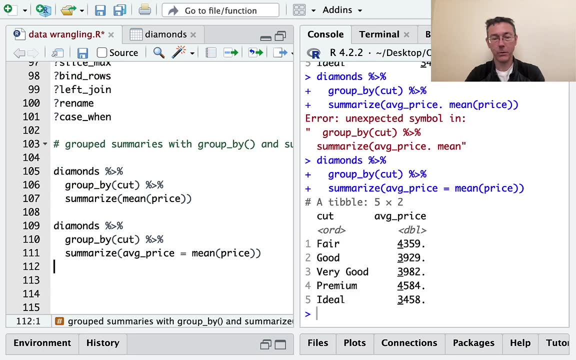 data frame and computed the mean price- Lovely. Now that doesn't look the best mean price as a column. Let's fix that. Let's call this column average price, for instance. Oops, I need an equal sign, not a dot. There we go. You can see, I got average price. We can do more than one summary. 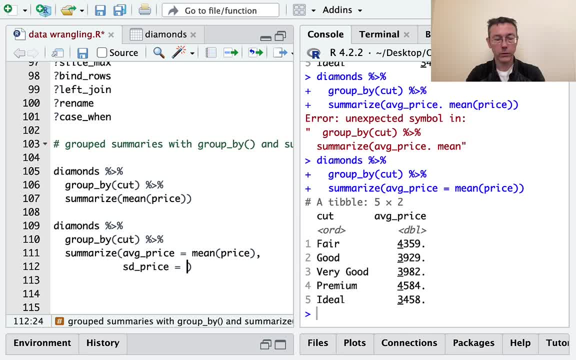 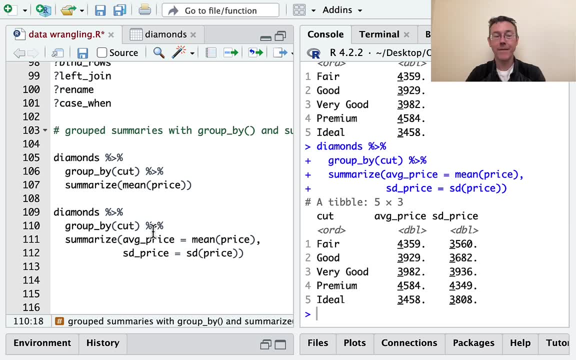 at a time. So we can, for instance, get the standard deviation of price, So that's SD of price. And there we got two columns in our output data frame. Fabulous: We can group by more than one thing at a time. 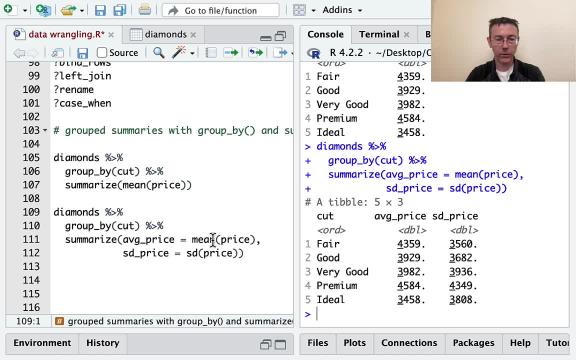 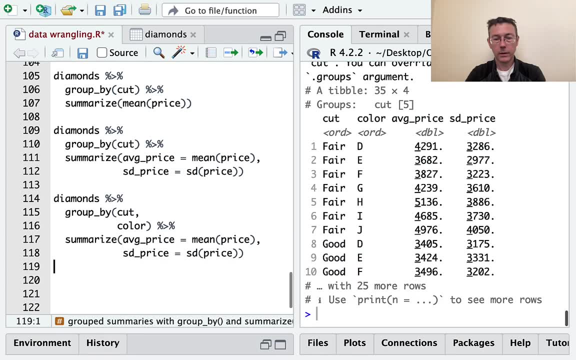 So let's see here- Maybe I'll just copy and paste this one- Let's break things down not just by cut, but also by color. Okay, So this is slightly larger. Now we have 35 rows And you can see that it is first grouped by cut. So I've got the fair cuts all together, then the good cuts all. 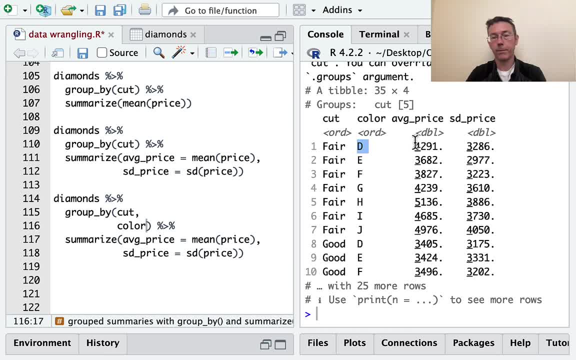 together, And then I've got the fair cuts all together, And then I've got the good cuts all together. And the second grouping is by color. And then it gave me those summary statistics for the sort of two-way table for the fair diamonds: fair cut diamonds of color D only. 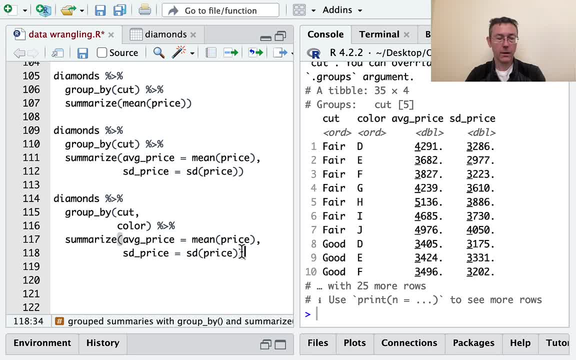 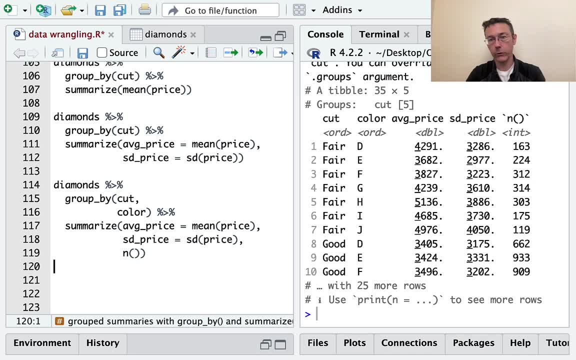 then for the fair cut diamonds of color E. only A very useful helper verb there when you're doing summary information is end parentheses, parentheses, And that just gives you counts. So here I can see there's 163 diamonds that are fair cut, that have color D. This is particularly 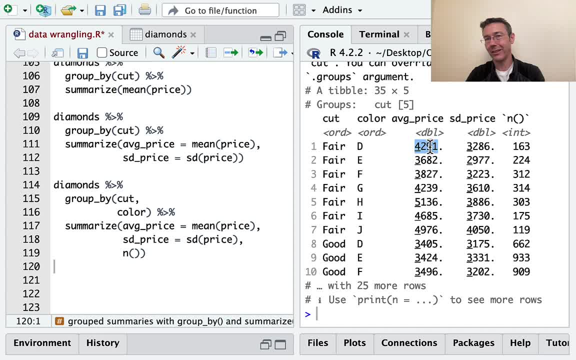 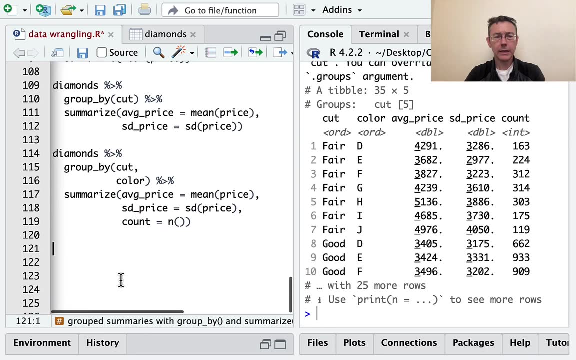 important because I'm doing these summary statistics. I don't know how significant or important, I should say, this average really is. Is that for a million diamonds? Is it for five diamonds? Makes a big difference. Maybe I'll call that column count. Okay, Sometimes you just want. 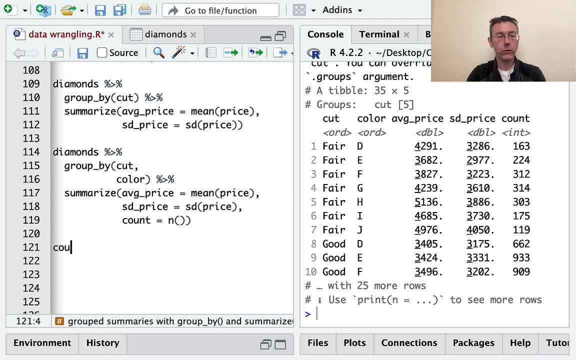 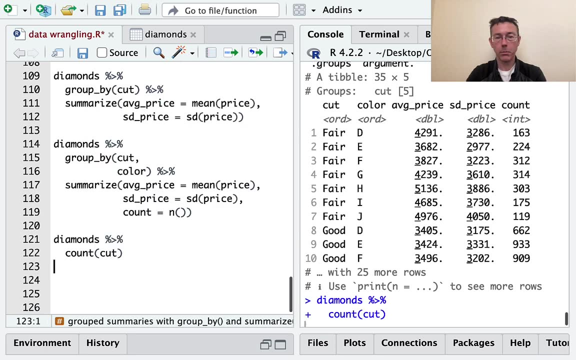 counts. You don't care about these other statistics in here And you can just use the count variable directly. So, to be consistent, let me use the pipe. I'll pipe diamonds into count, Like so, And now I just have to say what I want to count by, So I could count by cut. 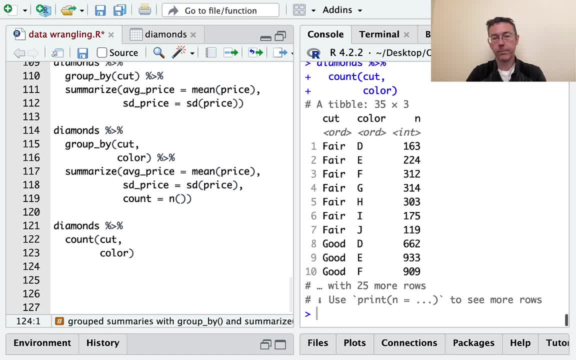 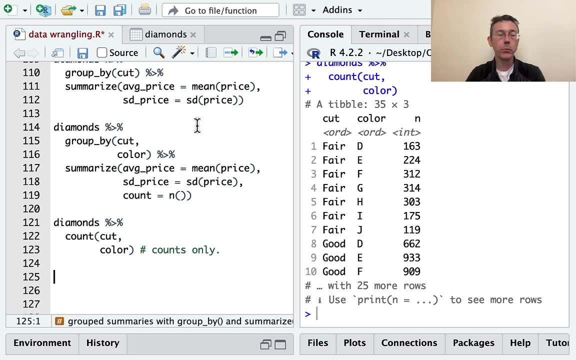 I can count by cut and color, So now I just have those ends. So let me just put a comment. That's counts only. Let's see, here I also can group by groups that I make up on the fly. Let me show you what I mean. So let me take diamonds. 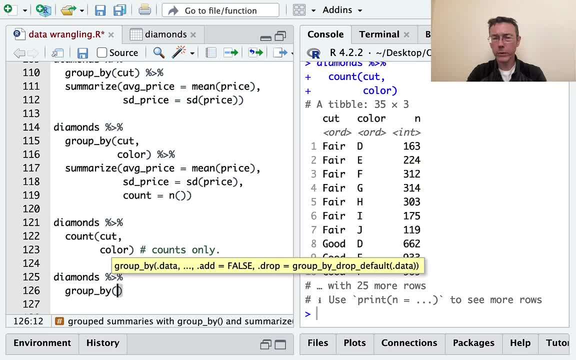 And I want to group it Now. I just want these expensive and non-expensive diamonds. Maybe. I don't want to create a whole column that says expensive or not. Let's group it by whether price is greater than 10,000.. Like so, And then I can do kind of the same summary as before, Maybe. 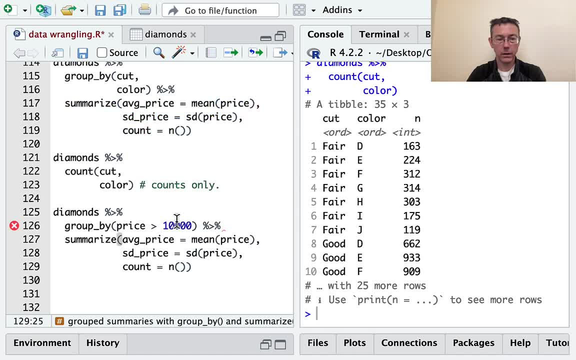 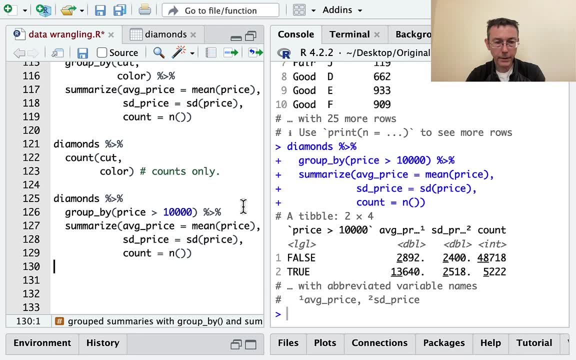 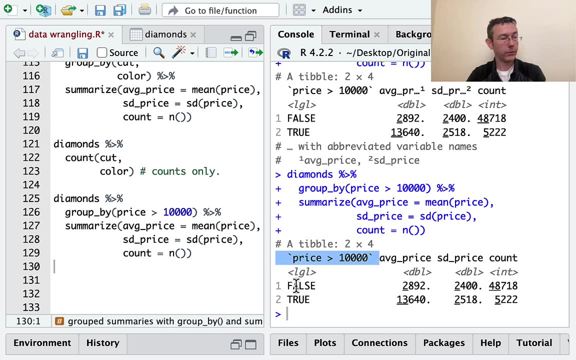 I'll just copy and paste that, if I can. That should work. There we go. Make a little bit wider so you can see it. So yeah, there we go. So now here's my group. I have diamonds that are not over 10,000.. I have diamonds that are over 10,000.. I have their average prices, and so on. 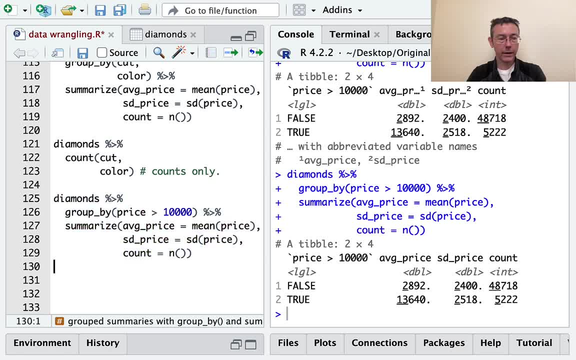 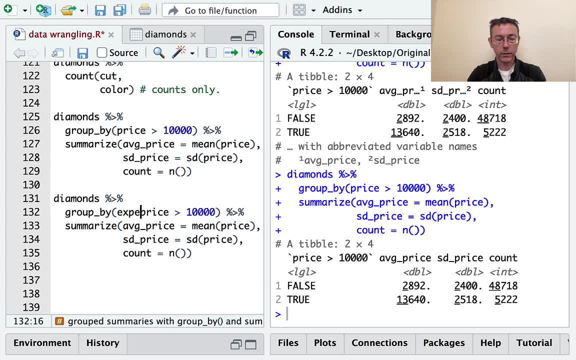 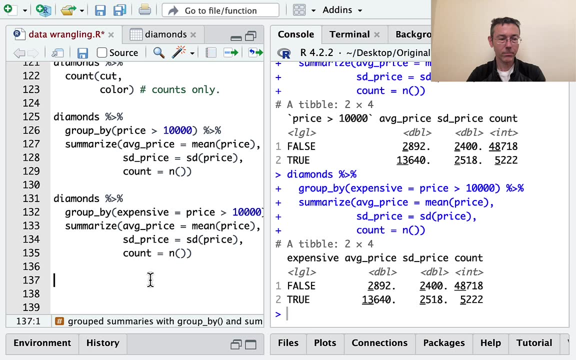 Nice, right. Next thing I want to do is to get a better column name there. So instead of price over 10,000, let's call it expensive And you can see. that fixed this column name right here. All right, I think that's good enough for a quick, rapid introduction to data wrangling in R using the. 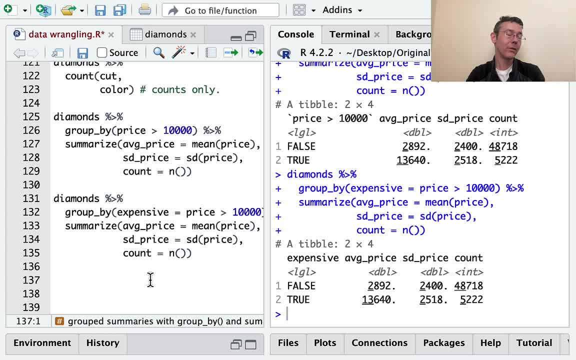 dplyr package. Like I say, I hope that you've gotten a bunch out of this And please check out some of my other videos. to go into these in a little bit more depth: 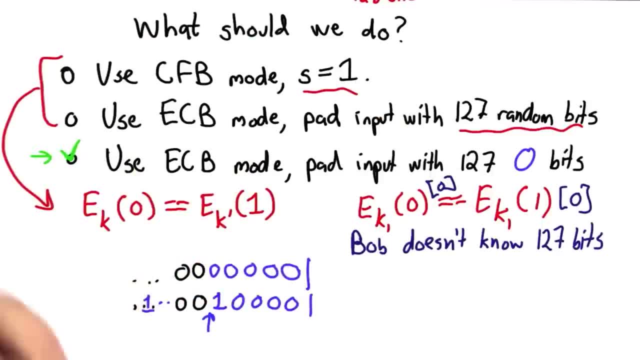 This approach works for the coin tossing problem, But there are lots of other situations where we need to commit to values, and we need to commit to values much longer than just one bit, And for that we need something a little more versatile, but with the same idea.